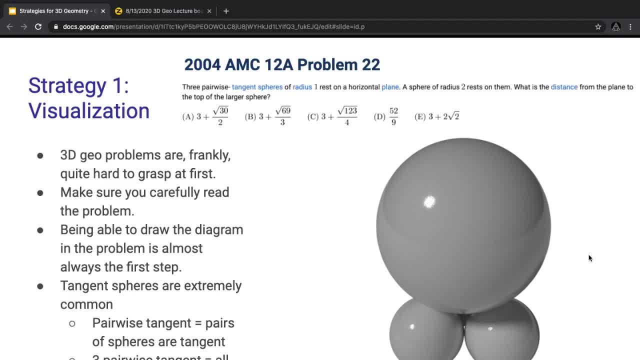 If you miss something, you won't be able to visualize it correctly, And being able to draw the problem is generally the first step. And because tangent spheres are extremely common, I'm going to just emphasize this point. So the word tangent just means touching at one point. Basically, if you look on the right-hand. 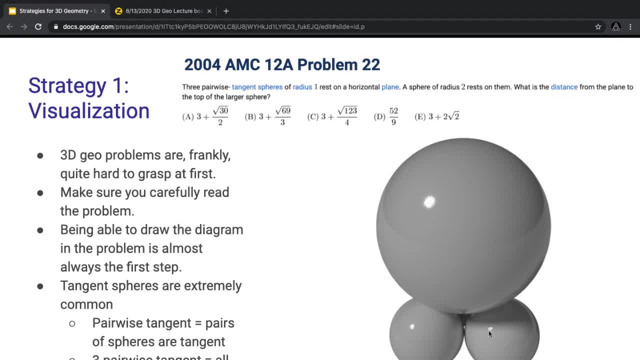 side. that diagram has tangent spheres at the bottom. Now if you have pairwise tangent spheres, that means they are tangent in pairs. So if you take any two spheres they should be tangent to each other. We also have three pairwise tangencies. 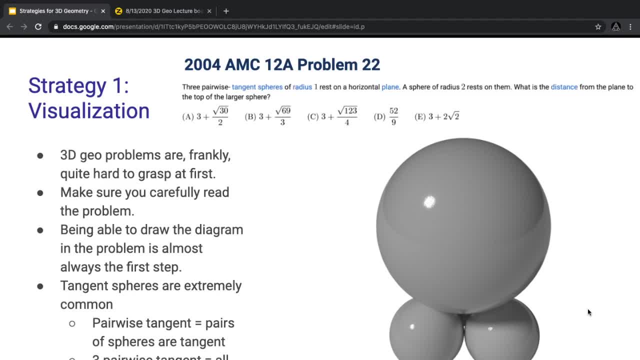 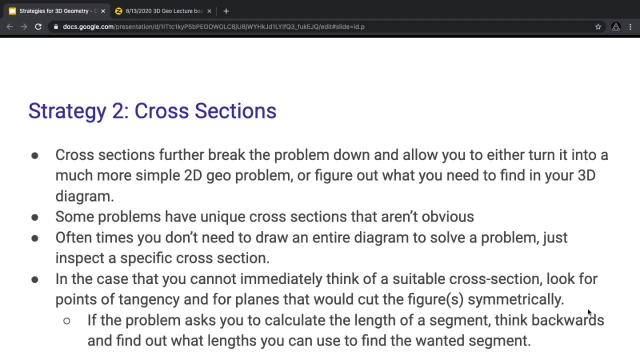 which means that all of them are tangent to each other, right? So yeah, We'll move on to strategy two. Strategy two is cross-sections. Now, cross-sections are extremely common, Like this is probably the most important strategy in 3D Geo. So cross-sections further break the 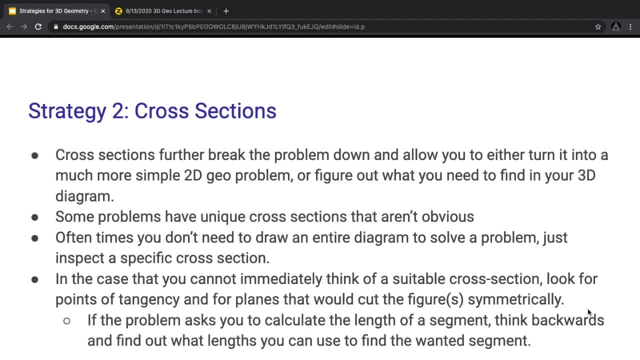 problem down and allow you to either turn it into a much more simple 2D Geo problem, or it allows you to fix the problems problem, or it allows you to figure out what you need to find in your 3D diagram. Now some problems have very unique cross sections that aren't always obvious and 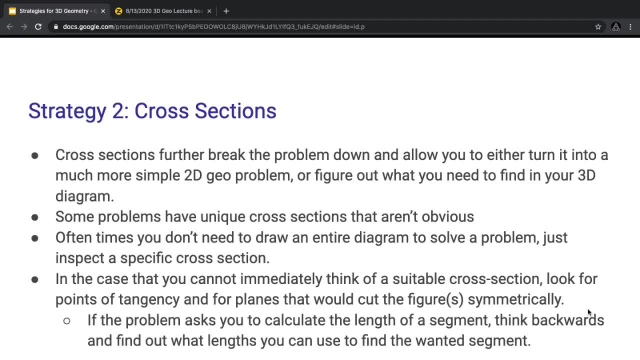 oftentimes you don't even need to draw an entire diagram to solve a problem. you just need to inspect a specific cross section. just make sure you pick a good one. Now, in the case you cannot immediately think of a nice cross section, you should be looking for points of tangency and for planes that would 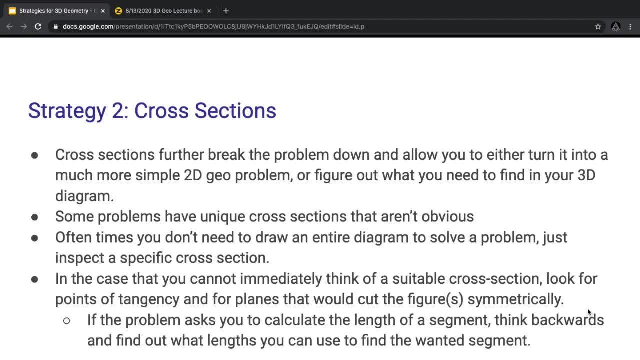 cut the figure symmetrically. so symmetry is like a huge theme, And if the problem asks you to calculate the length of a segment, I recommend thinking backwards and finding out what lengths you can use to find the wanted segment. so that's pretty good. So I have two example problems for cross sections. 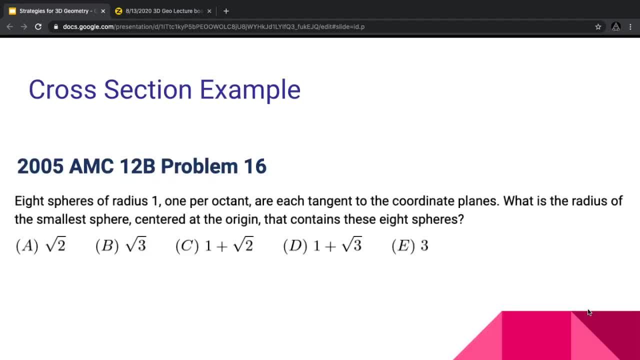 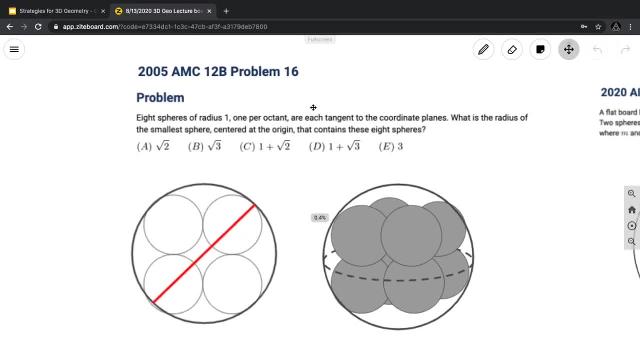 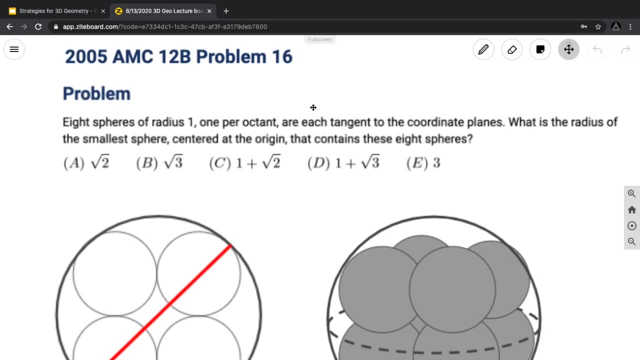 although cross sections are common in like every problem. Now, the first one comes from the AMC 12b, and I'll go right over to my whiteboard. Alright, so the problem reads: 8th sphere. So now the most important things to observe are that they're located one per. 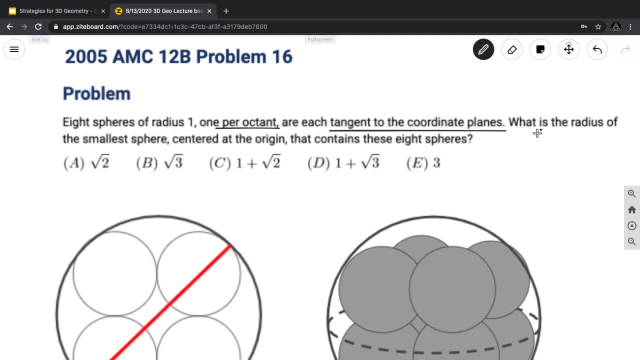 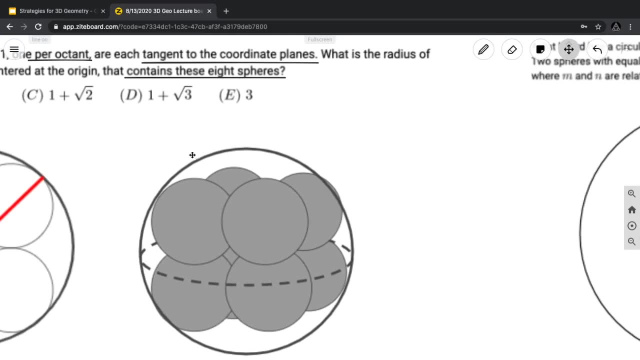 octant and they're tangent to the coordinate planes, and you want to find the radius of the smallest sphere that can contain these eight spheres. So first let's talk about the orientation. So right here I have a diagram like a quick visualization sketch. 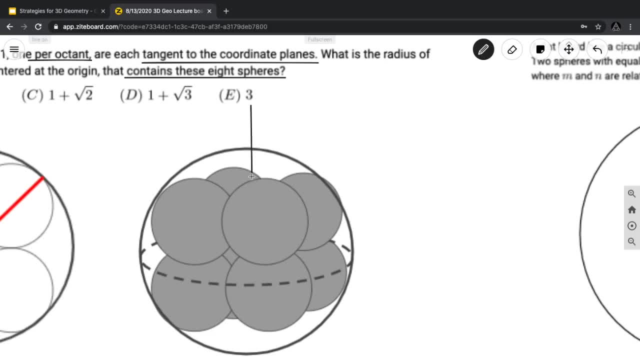 So how I got there. if we imagine the coordinate planes like- I'll try to draw it realistically or as best as I can, So the coordinate planes like the 3d Cartesian coordinate axes, they're gonna look something like this, right, So it. 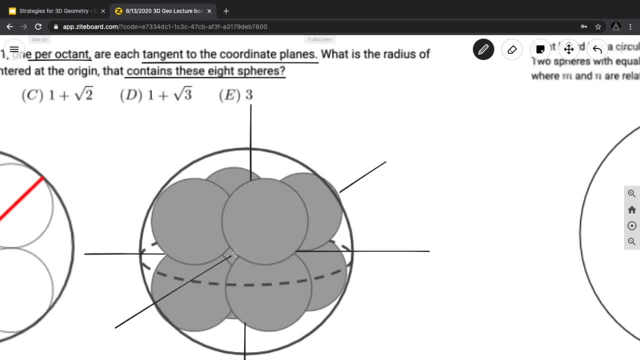 maybe comes out on the end. Now, in the middle you can't really see it, but like there's a area of intersection And these spheres, as you can tell, they're like, located one per eighth, like, so each sphere takes up one eighth of the entire. 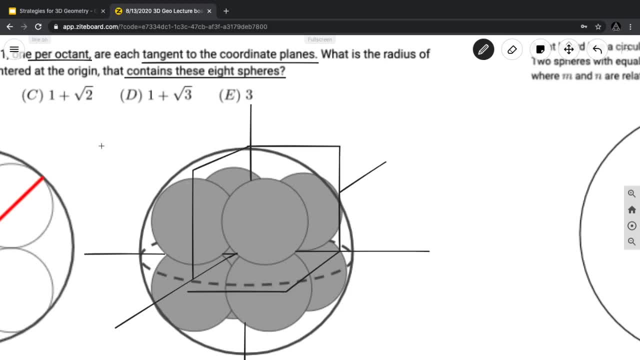 coordinate system right, So they're located per section. That gives us that 2x2x2 setup. Alright, I'll get rid of those lines. And now we also see that the largest sphere that can contain these eight spheres, well, the smallest sphere that can contain the 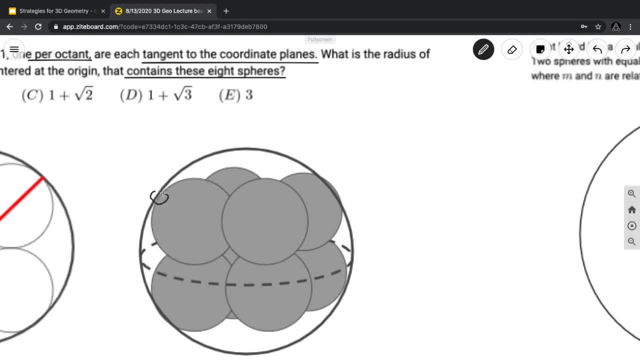 eight spheres. it should be tangent to those spheres. So you see a tangent point here. there would also be a tension point maybe here here, one at the bottom. There's going to be one tension point per sphere. That gives us the smallest. 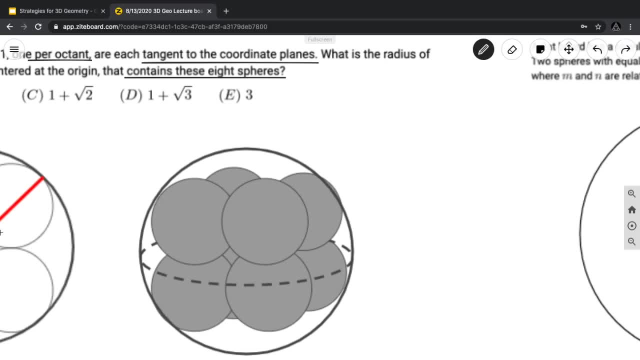 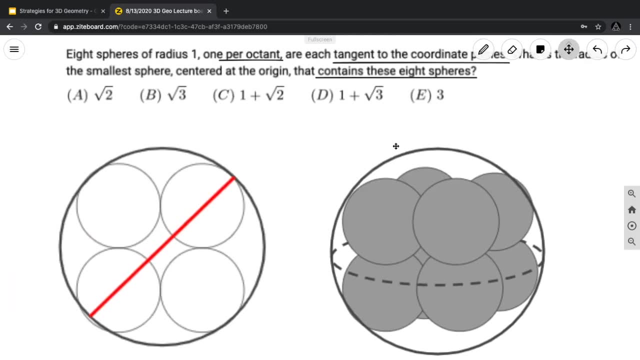 possible one. Alright, so with the configuration and the diagram in mind, we can move on to the cross-section. Now, the cross-section we want to take here is kind of unusual. Basically, the diagram on the left is actually an aerial view of the diagram on the right, So if you're 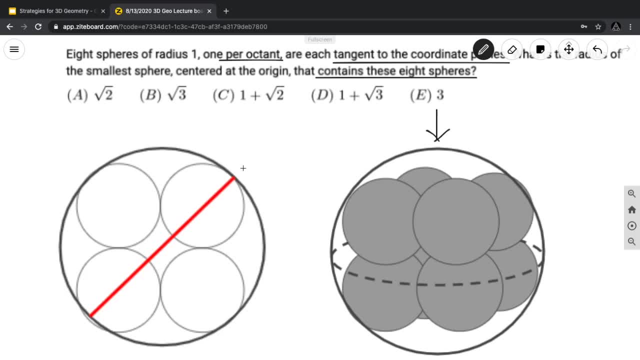 looking from the top, what I want you to visualize is this red line. That's what we're gonna cut at right. It's a cross-section. you like, cut the diagram to make it. And this cross-section what it does. like if we 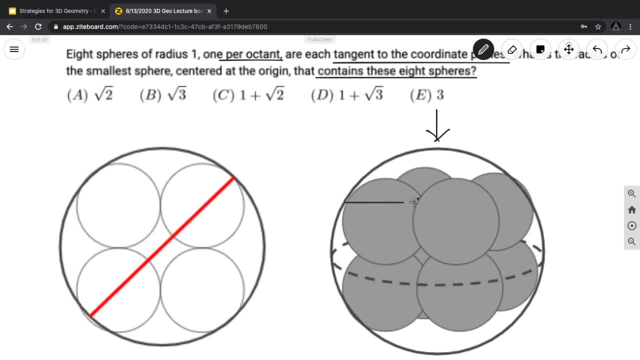 just visualize it over here. it's basically sorry, it's basically this line And it cuts like this plane. So you might be wondering why right? Why would we ever choose this cross-section? The reason is because when you cut it and you break, 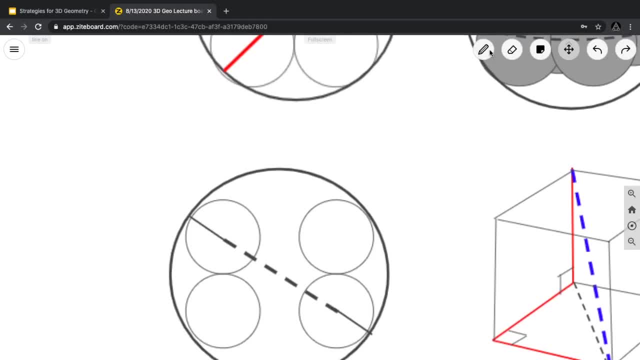 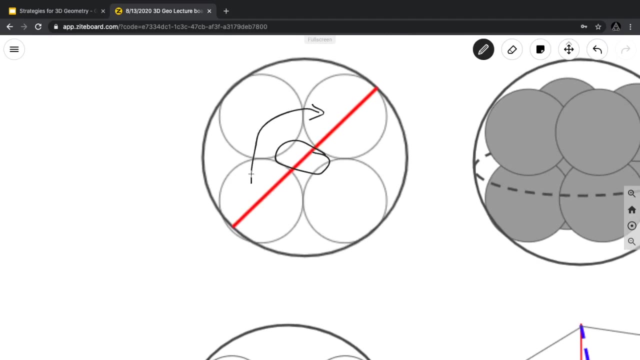 open the sphere, you get something like this. And this diagram is quite unusual because you might be wondering what the gap is doing here. So why is there this gap between the spheres? right, That is because, if you look at this gap in the center, that's because these two spheres are not tangent to each other. 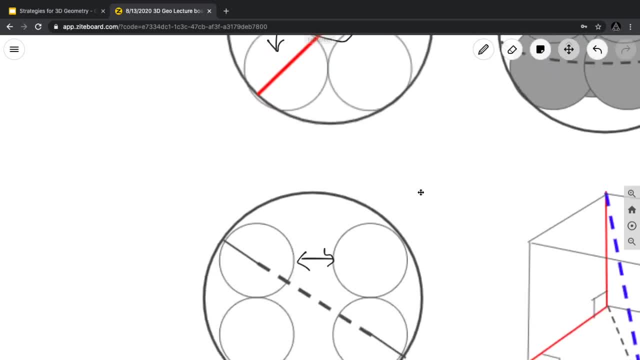 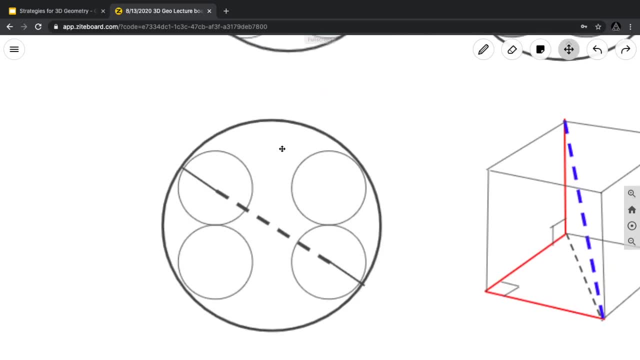 They're opposite from each other. that gap is reflected down here as well. Okay, now moving on to the actual like solving. So, with this in mind, we want to find the radius of that large sphere right, And to do that. 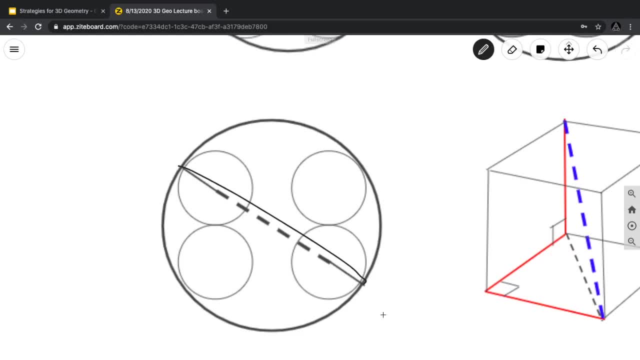 we can actually just find this diameter first. This is the most important thing to find, And through later observations I'll just quickly skim over. for now you can observe that this line will go through the centers of these points. That's very, very important, because that means 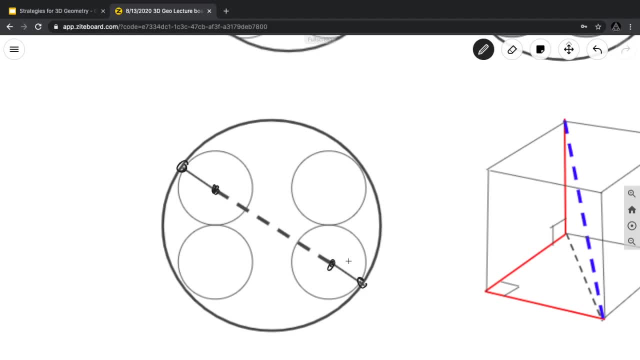 we can split the segment into the union of three separate segments: right, And the radius here is one, and the radius here is one. So what we really really are left to find- whoa, what we want to find is actually this: the length of the middle segment. Now, how do we do that? right, So, 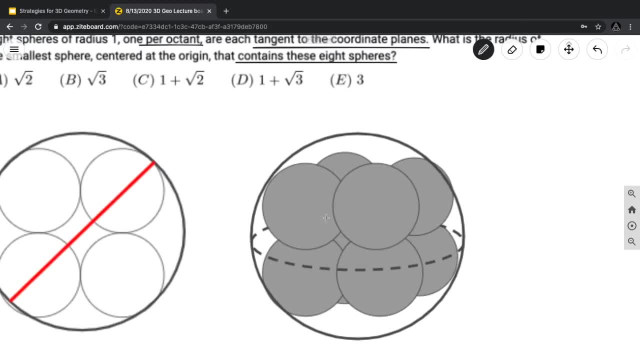 first, we want to observe what the middle segment is in the actual diagram. So if I consider this one and this one, basically the middle segment is this length. Now, the key to finding the length is to find this вокруг. Therefore, Candimo really wants to find that middle segment. 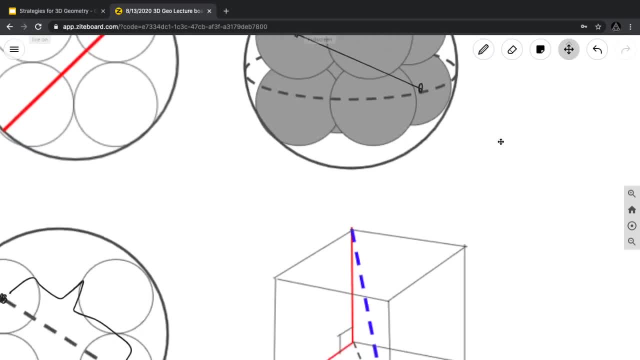 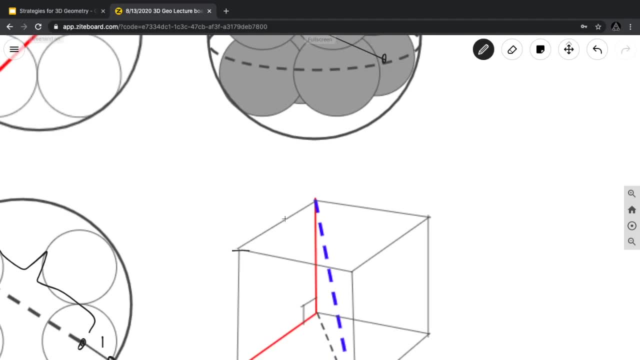 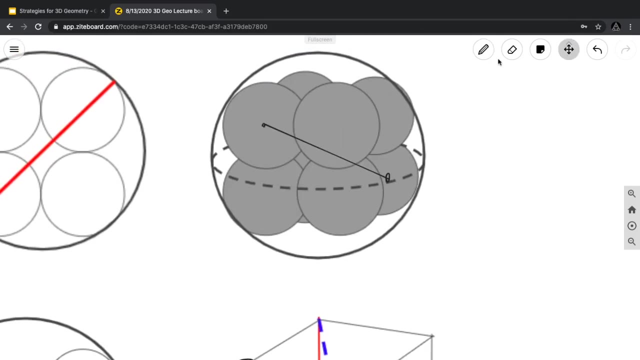 length is actually to draw a diagram of all the centers of the circle. So basically, in this cube, every vertex is going to be a center of a circle. So this is going to be a center of one circle- well, one sphere, sorry about that- and a center of another sphere. And why is this true, If you? 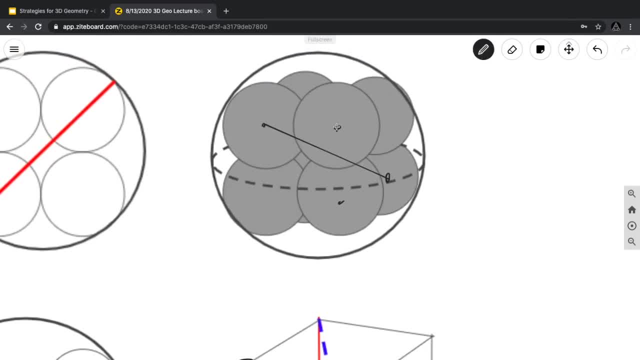 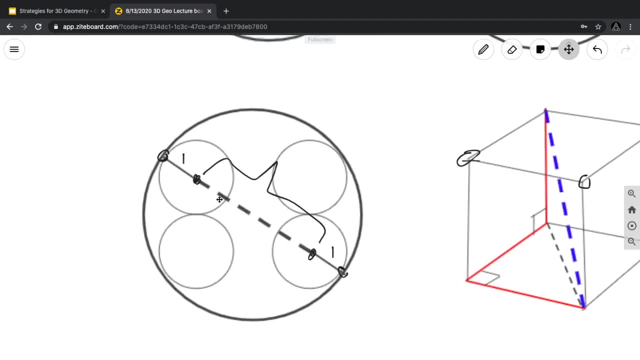 just observe, we see that it creates a square, and then the square becomes a cube when you connect the other vertices. All right, so with that in mind, now we want to find the length of the dotted blue segment, which is the same thing as this dotted black segment, And from here on out, 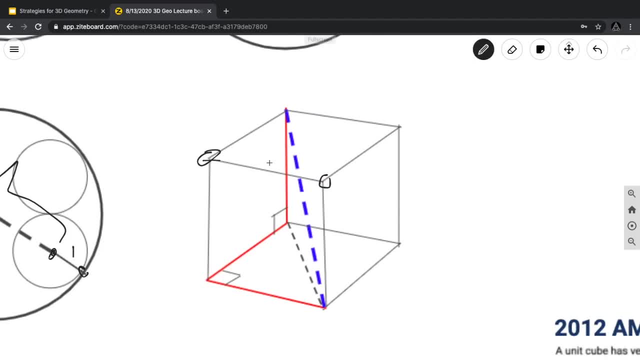 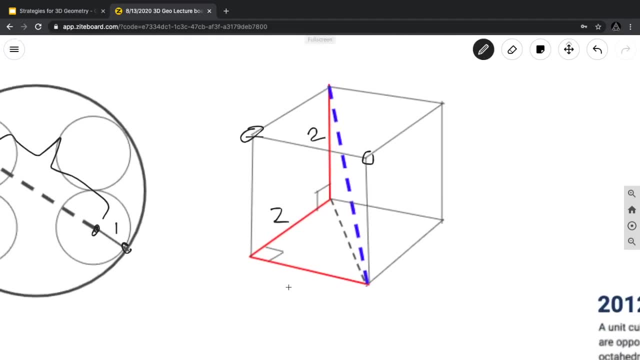 it shouldn't be too hard. All right, so what we have to do is: we know this is 2, because it's the union of two radii, and each radius has a length of 1.. Now 2,, 2, and 2,. this is a 45-45-90 triangle. 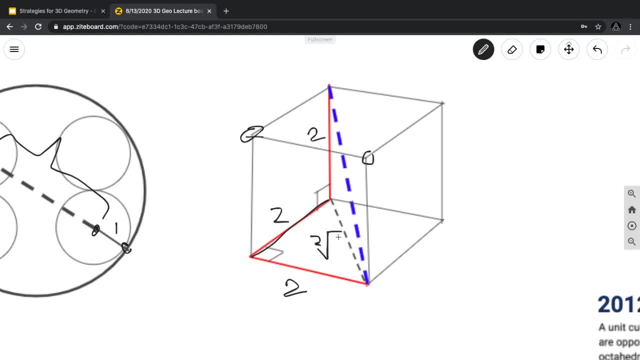 down here. So then we know the hypotenuse has a length 2 root 2, and we know that the length of 2 root 2 is 2, which is the length of 2 root 3.. So we say we know that first we have. 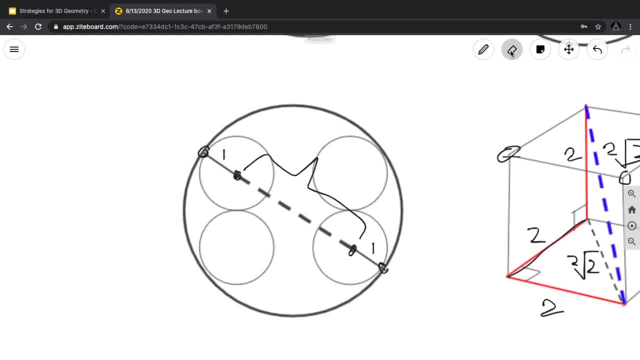 the right layer, or the Очень tunes. So the new diagram we're going to take here is that the frontal joint of our triangle pieces is 1: 1, 1, root 2, and now we know that the horizontal, since these two sides areะ our left and our right sides, are modeling it the same way which we do, because we understand this relationship. And then I'll go over here again: immense gradient, more diagonal or even a Mongolian diagonal. So if you want to figure it out and develop your equations using these two equations, now I'll let you focus in on there, But first I want you to 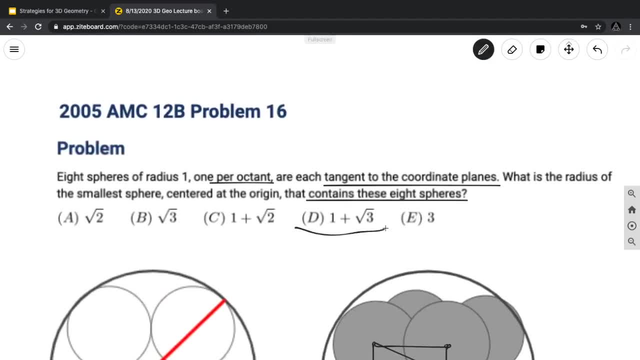 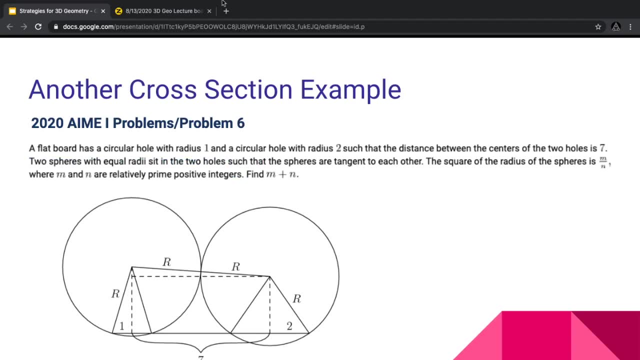 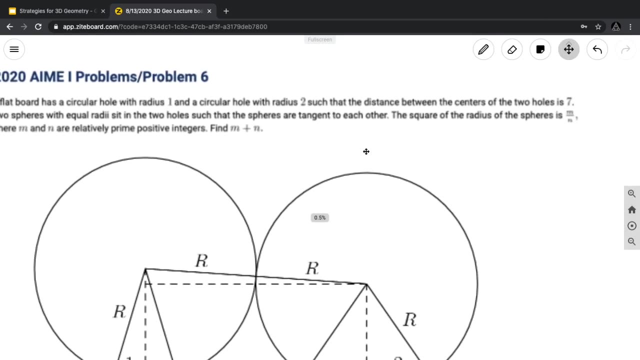 as our final answer. so our answer would be D. All right, so our next problem is an Amy problem from the 2020. Amy I and I'll go right back to the whiteboard. All right, hopefully everyone can see this clearly. So it reads: a flat board has a circular. 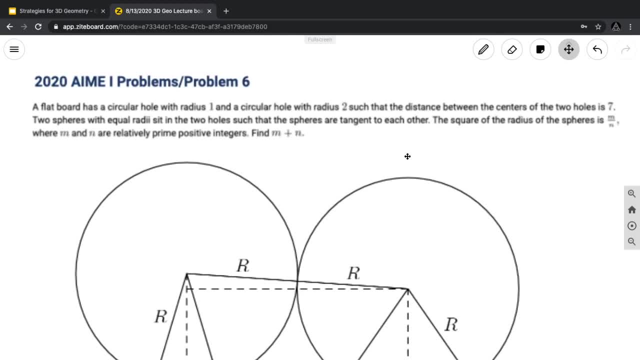 hole with radius 1 and a circular hole with radius 2, such that the distance between the centers of the two holes is 7.. Two spheres with equal radii sit in the two holes such that the spheres are tangent to each other. The square of the radius of the spheres is m over n, where m and n are. 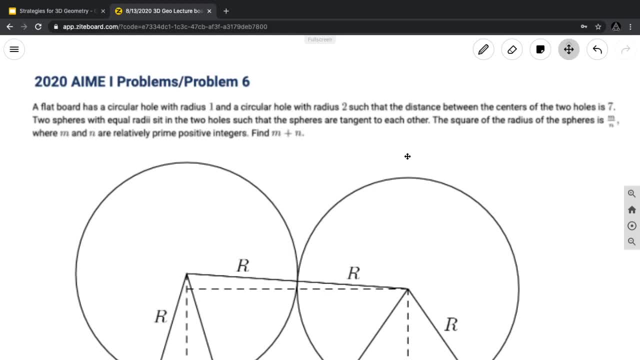 relatively prime positive integers. so find m plus n. So first two notes. I forgot to mention this earlier. we're going to plan on ending at around 8: 45 pm Eastern Standard Time, so just keep that in mind. And also, if you're not familiar with the setup of the Amy, all the answers to Amy are: 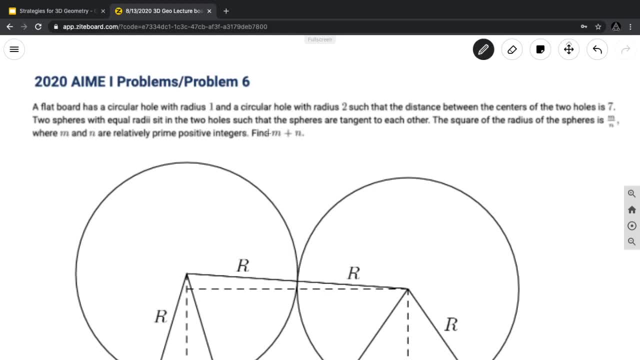 integers from 0 to 999.. So that's why it says like find m plus n. because you can't, it's just not possible to input m divided by n, because it's the Amy and that's the nature of the test. So, going on to the problem, 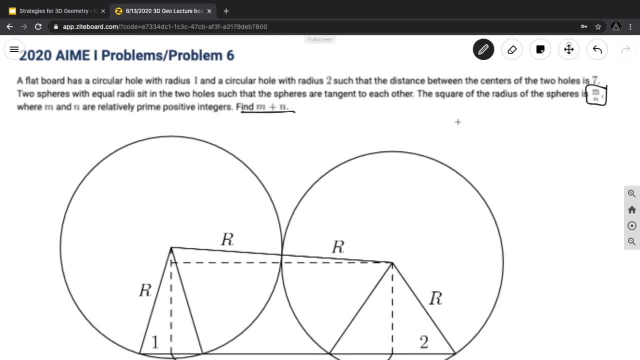 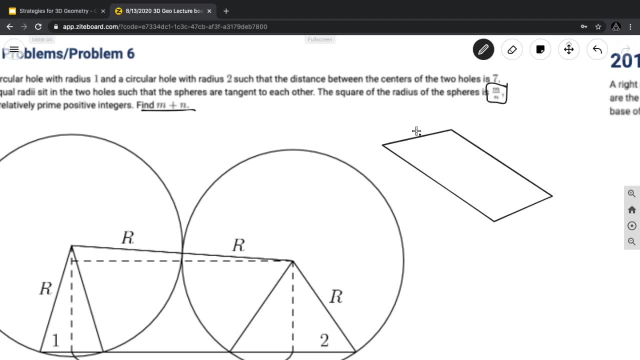 right here. I already included the cross section. However, if you guys want to just like see the visualization, it looks something like this: Basically, we have that flat board and then we're going to have two circles, So maybe one here and one slightly lower. Now these circles: 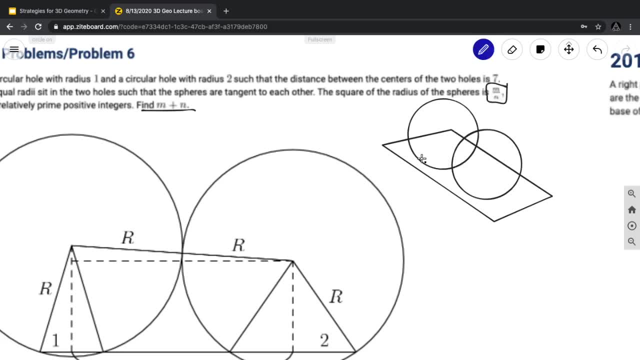 have equal radii, just keep that in mind. And these circles sit in two circular holes in the, in the like oops in the floorboard. So what that looks like, maybe one sits like this high, but the other, like the other hole, is much larger. 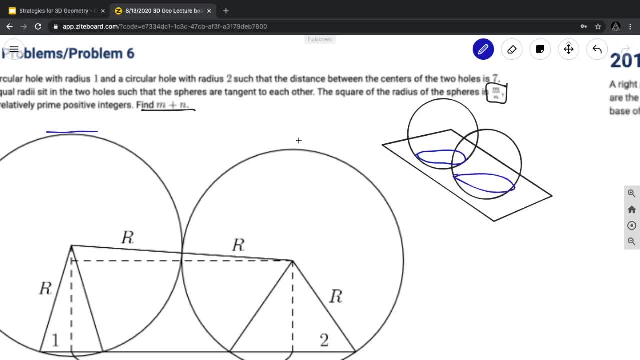 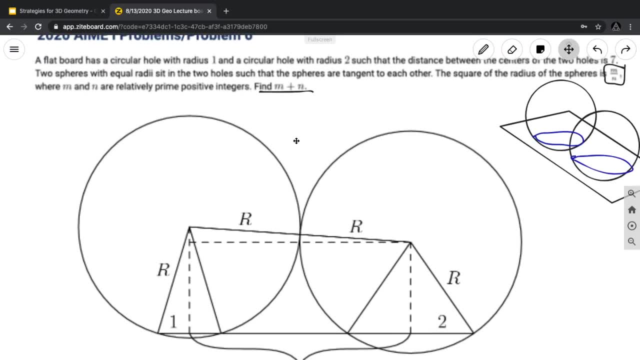 So what that means is that there's going to be a height difference between these two spheres. there's like a pretty large gap. Now, that's what makes this diagram kind of unique. Okay, so, with the cross section in mind, what this cross section is going to do is it's going to 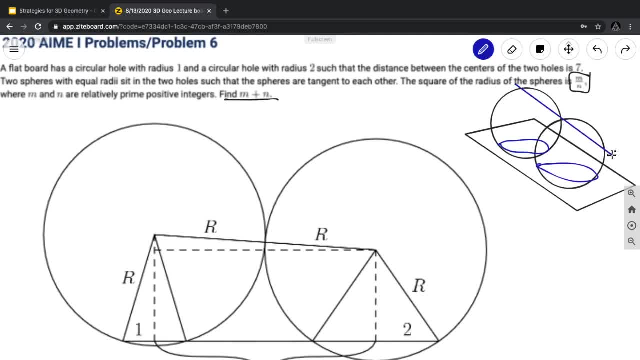 actually is. it's just a straight line that cuts right through, like it cuts right there. So this is definitely will this definitely will include that tangent point which is so crucial to our problem because it allows us to connect, like, in a way, it allows us to connect those two spheres. 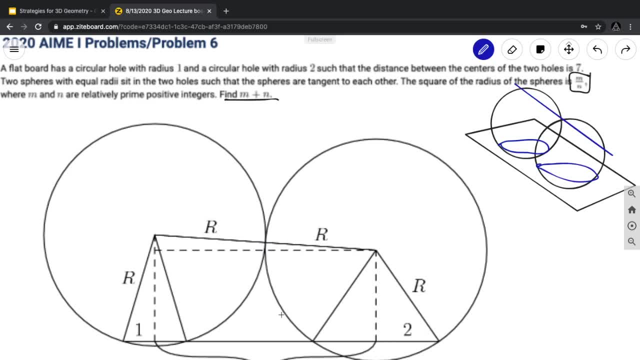 pretty important. Now, moving on to actually solving. So we want to basically create an equation that allows us to solve for r, which is the radius, And we notice a really useful right triangle up here. So this right triangle is what we want to take advantage of. It's a right triangle because the height is inherently 90 degrees when you consider parallel lines. Now, 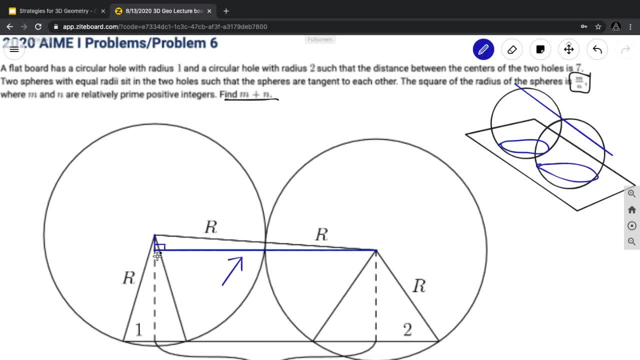 we already know what this is. this is just seven, right, Because we have a rectangle, So that length is already solved for. However, to find the small height, what we want to do is actually just take this height and subtract it from this height. Well, to subtract the second height from the form. 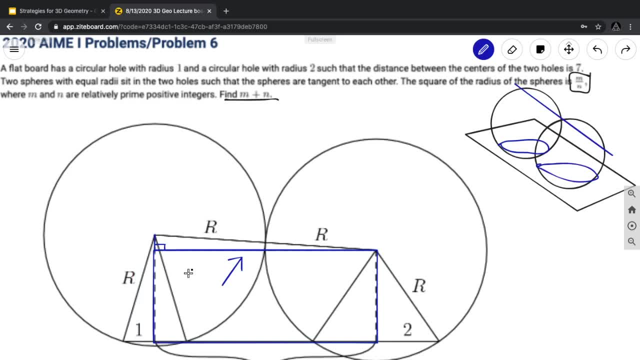 we're going to use the Pythagorean theorem Now. to do that. you would just use some basic Pythagorean theorem. Pretty simple, yes, You just take the square root of r squared minus one- excuse my poor handwriting, sorry about that- And then we'd subtract the other height, which is r squared minus two squared. 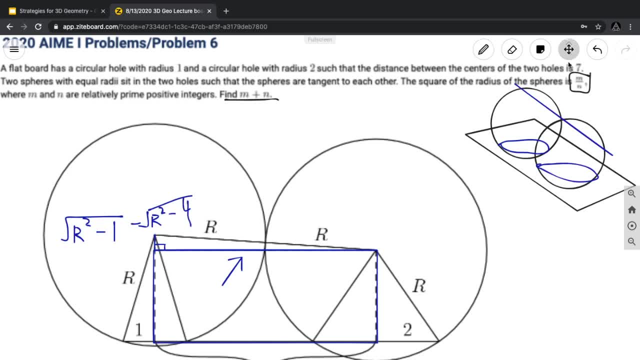 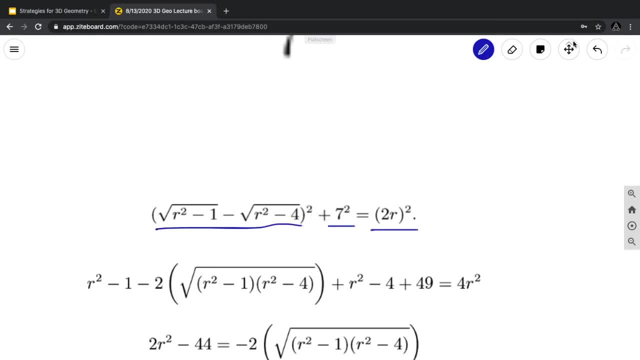 which is just four. Now, with all our side lengths, we can create an equation which is right here. So here's one leg, here's one leg and here's the hypotenuse, And this is just the Pythagorean theorem. 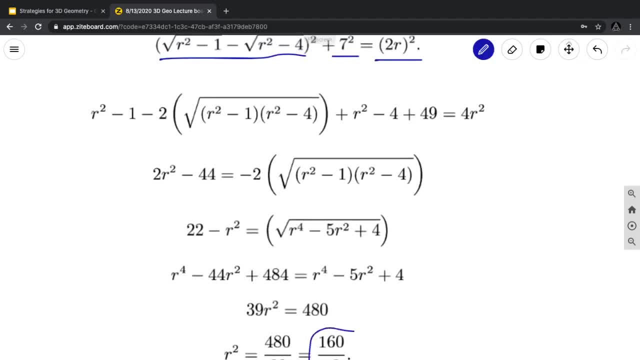 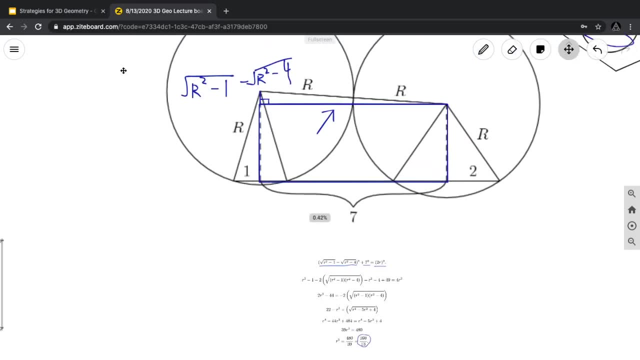 And when we solve, we find an answer of 160 divided by 13.. And if we add the numerator and the denominator, we get a final answer of 173.. All right, so with that out of the way, let's move on to our next strategy. 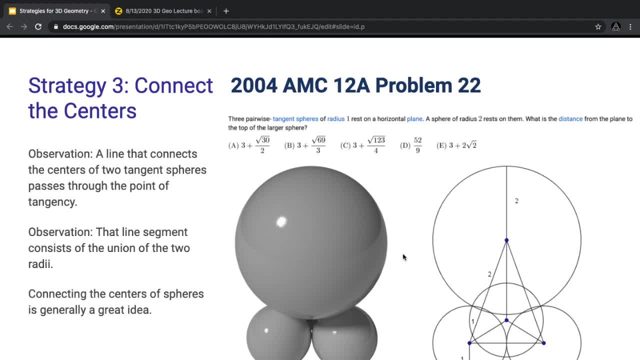 So strategy three is connect the centers. Now, this is a very common strategy actually in Euclidean geometry. However, it applies even more in 3D Geo, because when you're dealing with tangent spheres all the time, which means you're going to want to connect the centers to create a good diagram. 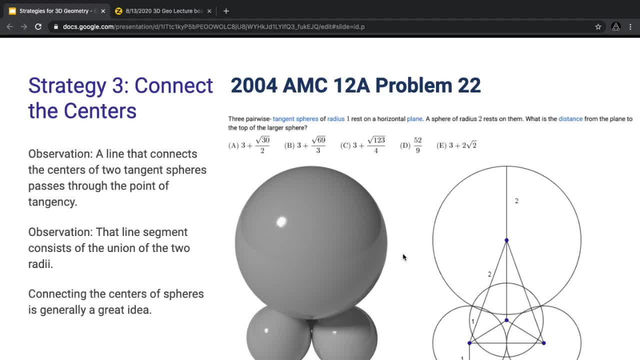 So an observation I shared earlier is that a line that connects the centers of two tangent spheres always passes through the point of tangency. This is important because it gives way to the second observation. It states the line segment. that line segment consists of the union of the two radii. 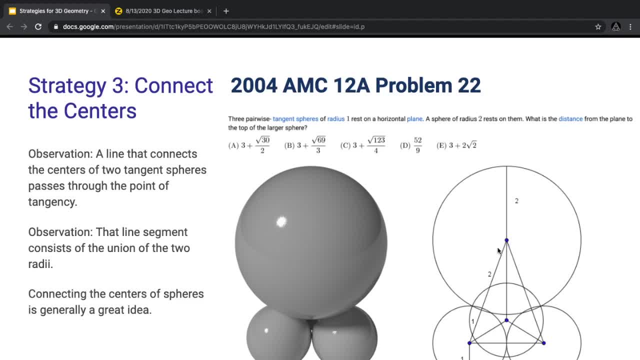 So that just means if you look on the far right diagram like this point connected to this point, the segment is just equal to one plus two because this segment passes through the tangency point. So you can just add up the two radii to get the length. 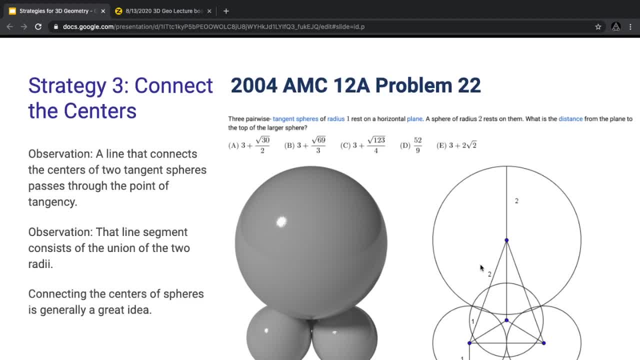 So this is why connecting the centers of spheres is a very, very good idea. All right, so if we wanted to actually solve the problem, this problem, what we want, what the question is asking, is basically the distance from the top of the second sphere to the plane on which the three pairwise tangent small spheres lie on. 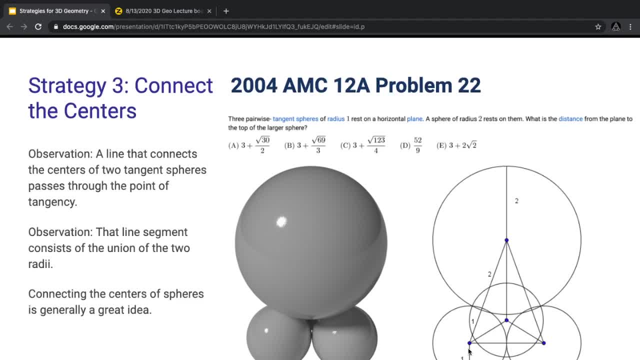 Now this height is actually just equal to the bottom radius one plus the top radius two, plus the height of the tetrahedron recreated by connecting the centers of the spheres. Now you might be asking: how could I possibly get the height of the tetrahedron? 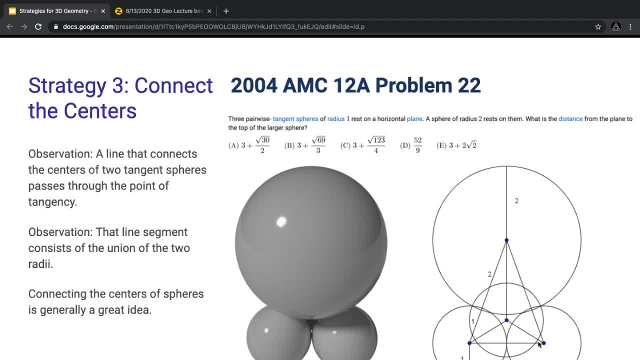 It's actually quite simple Because we observe the bottom equal. the bottom base is an equilateral triangle. then you're able to pinpoint the center of the triangle by using the property that the distance from the center of the triangle to a vertice would just be two-thirds of the height of the equilateral triangle. 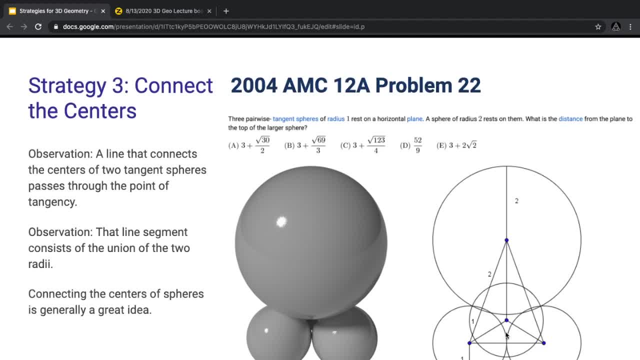 I won't actually solve it right now, but that's the outline. And then you use Pythagorean theorem to get the height and you add it all up. All right, so if you look at the answers, you'll see a lot of three plus something. three plus something. 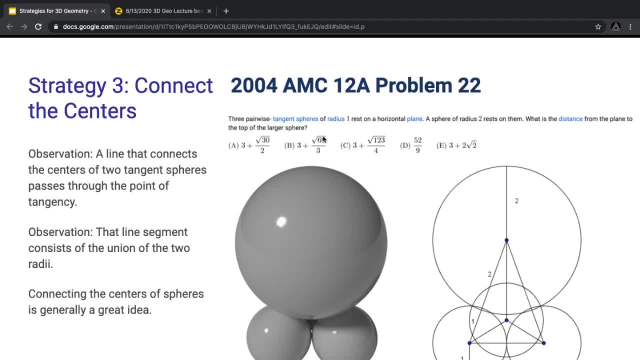 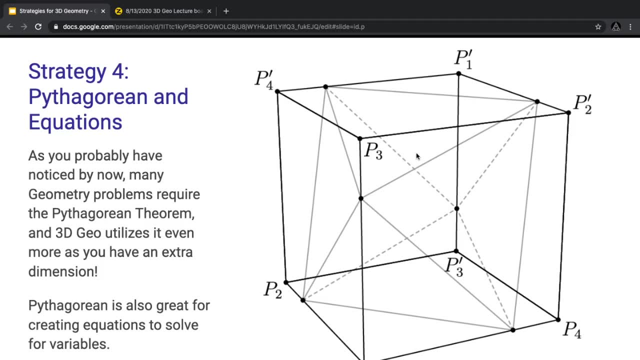 That's because you add radius two and radius one to the height and the height is definitely a funky like square root. All right, so strategy four is Pythagorean and equations. I'm just gonna drink some water real quick. 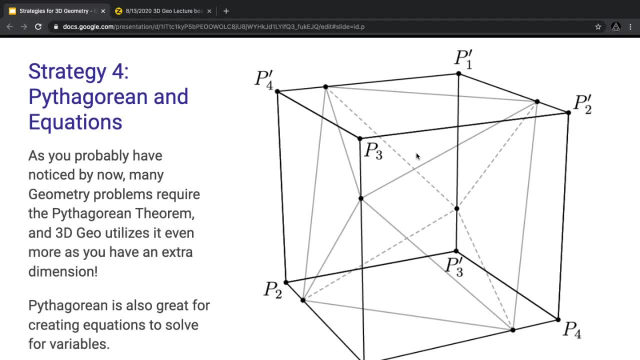 All right. so, as you might have noticed by now, like a lot of 3D, Geo problems require a ton of Pythagorean theorem. That's probably because you have an extra dimension to contend with. right, It's 3D instead of 2D, But Pythagorean is great because it allows you to create equations to solve for variables. 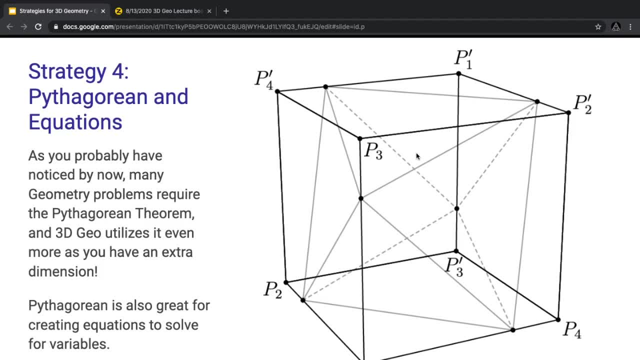 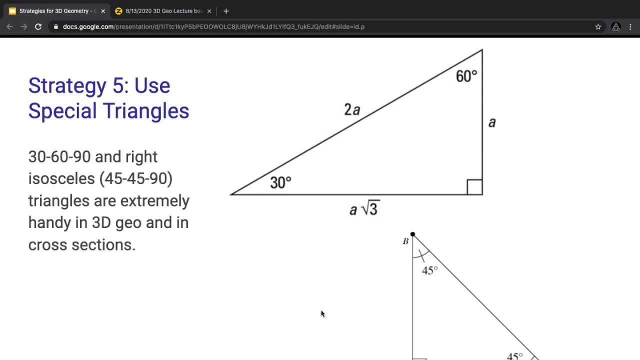 So earlier we had a problem that required that, and I'll just do another one later. Nothing much too much to say about this one. Strategy five also applies in 2D Geo. It's using your special triangles, So you should, you guys should. 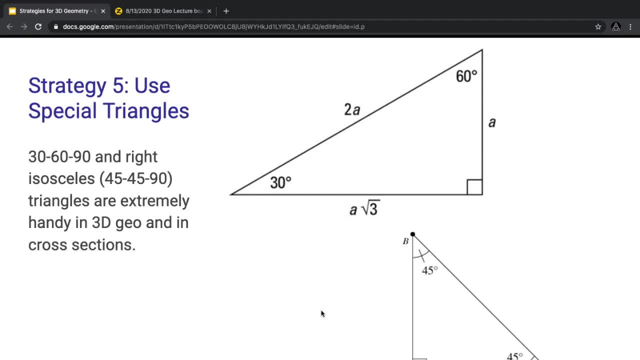 uh, know these if you're at the AMC 10 level. If you're not familiar, basically we have two very unique triangles: the 30-60-90 triangle and the 45-45-90 triangle. Now, these are unique because, one, the angles are easily identifiable and, two, their side ratios are determined. 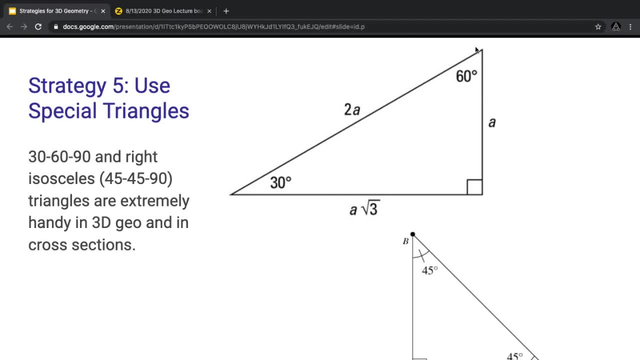 Basically a, a root 3, and 2a are the ratios of the side lengths and in the 45-45-90 triangle you're gonna have 1, 1 root 2 as the side length ratios. and that is because 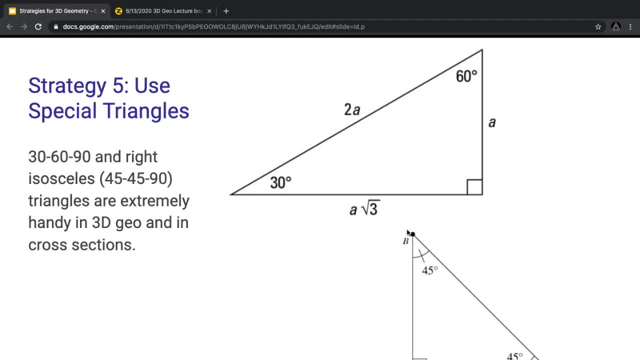 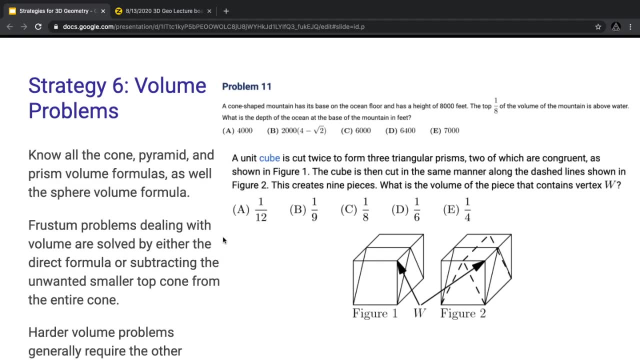 this is a right isosceles triangle. You can verify all of this just using the Pythagorean theorem. All right. strategy six deals with volume problems. So, first and foremost, you should know all your cone, pyramid and prism volume formulas, as well as the sphere volume formula. 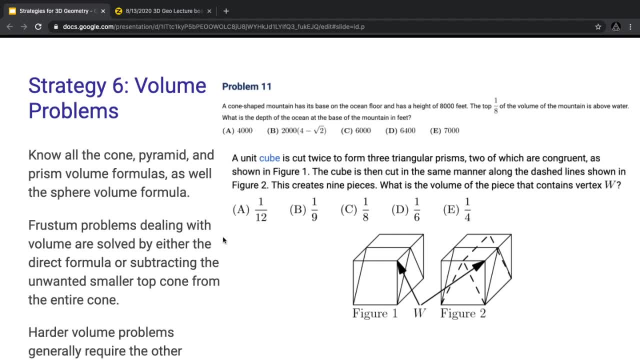 So all of these are extremely important, but you could Google them if you're. if you need a refresher Now, what is a frustum? A frustum is basically a cone with a top portion cut off, So you would imagine it's like a conical trapezoid. 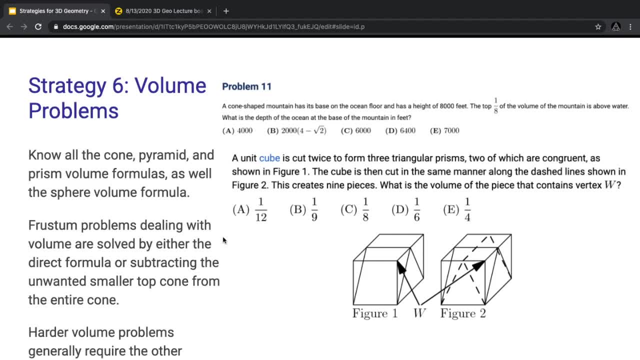 Frustum problems. deal with, uh, dealing with volume, like they're really annoying. if you do not know the direct formula for the volume of frustum, Or so, the only other option would be to subtract the volume of the smaller top cone from the entire cone. 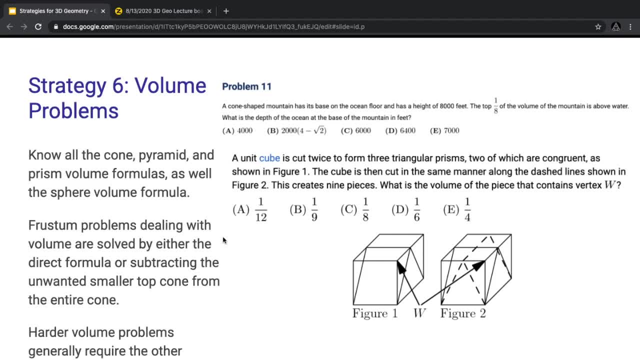 But harder. volume problems generally require all the strategies in conjunction. So let's quickly do these two problems. The first states a cone-shaped mountain has its base on the ocean floor and has a height of 8,000 feet- The top 1 eighth of the volume. 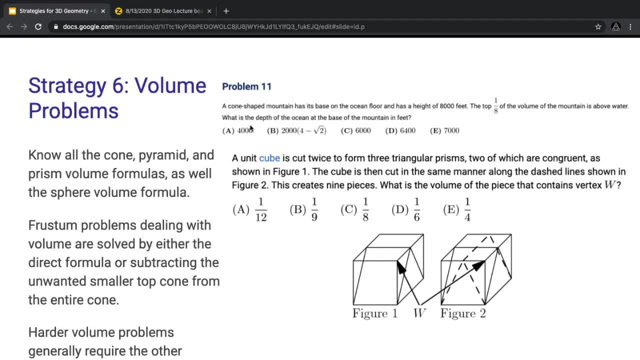 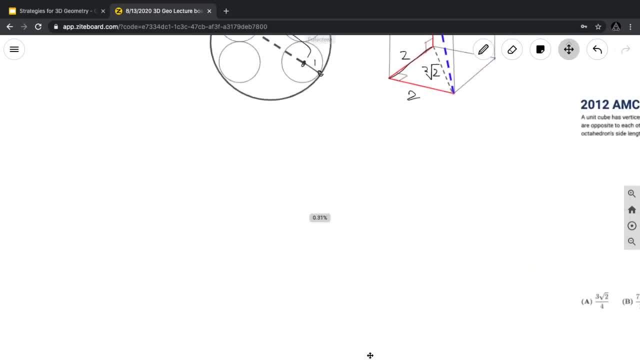 of the mountain is above water. What is the depth of the ocean at the base of the mountain in feet? So let's go over to our whiteboard, Alright. so let's just do a quick sketch. So maybe here's the ocean floor and then we have our conical mountain. 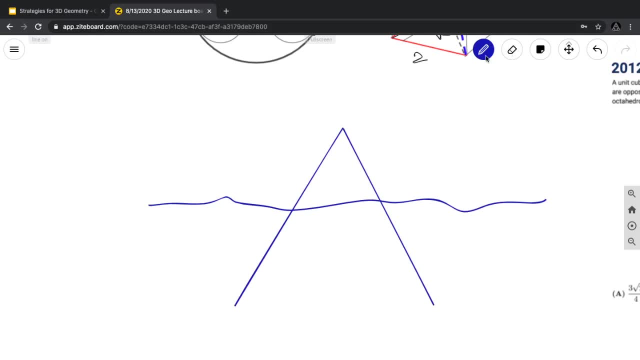 So here's one side, here's the other side, And then we have our base, which is: it's a cone, And the only thing other thing it gives us is that the height is precisely 8,000 feet. 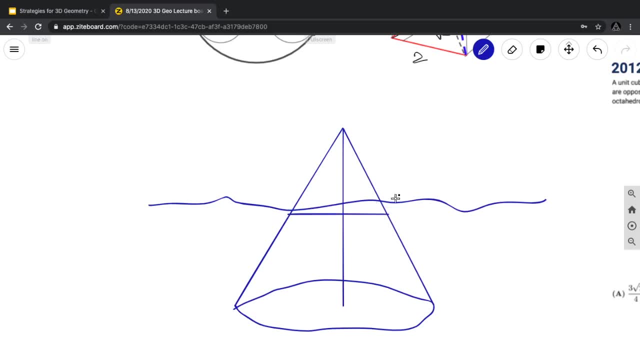 Now let's just draw a straight line for clarity's sake. That's going to be the ocean level, Alright, so what we want to do is identify the bottom portion of the height, which I'll outline in red. So we want to find the red section. 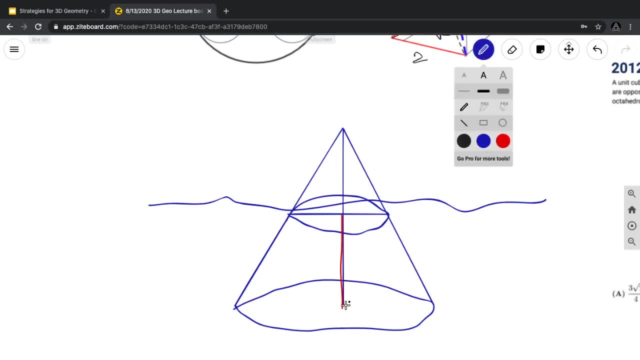 Okay, so how do we do this, You might be wondering. It's actually quite important. So the most important observation to make is that volume and side ratios are inherently connected. If you just take, you can verify this in a few minutes. 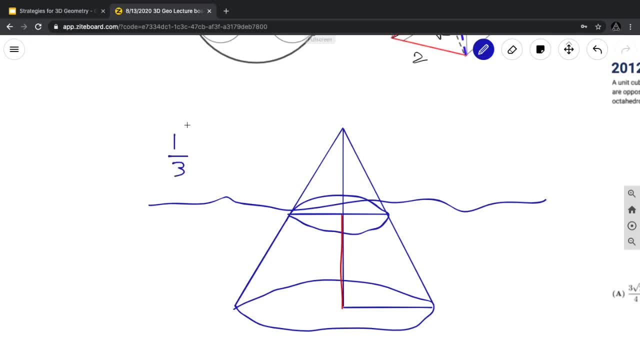 If you just take like, let's just say there's a ratio of 1 to 3 for side lengths. If you directly can connect it to a volume, you can just take the cube and the ratio of the volumes would be 1 to 27.. 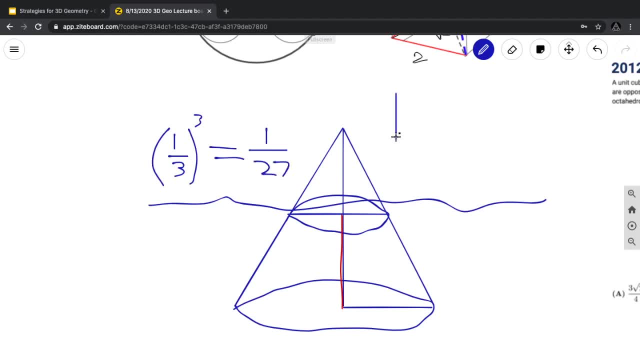 I'll illustrate this with another example. Let's say you have a unit cube, right? So that unit cube is going to have, maybe, side length. it's going to have side length 1. Alright, and then if you want to find like a unit cube with all of side lengths 1 half, 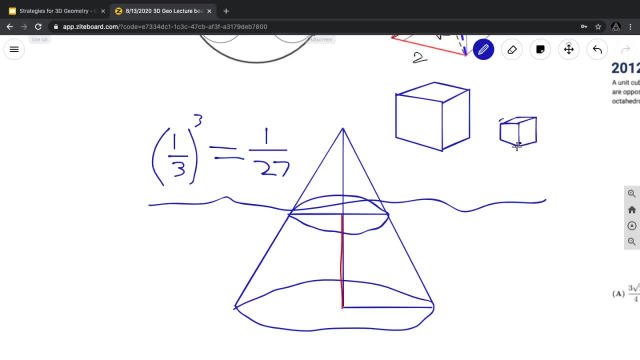 it's quite simple to observe that this unit cube, its volume is 1 half of the other, of the larger unit cube. That's just because the side lengths- there's 3 side lengths in ratio and when you multiply all the side lengths together that means you're cubing the ratios. 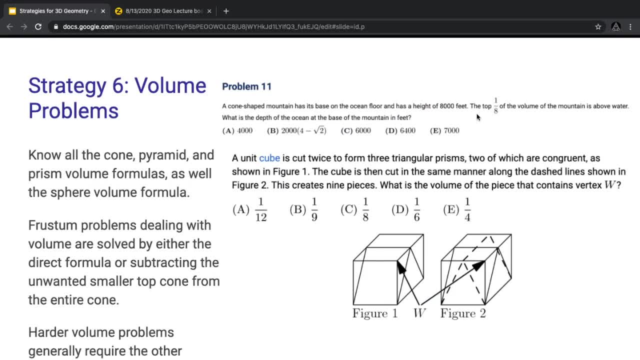 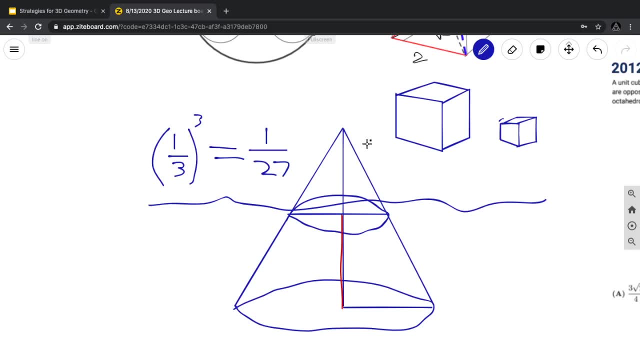 So, with all these good observations, let me just check the problem. It says the top 1 half of the volume of the mountain is above water. So that just means we have 1 half of the mountain above water. and if you consider the side length ratios, because these two 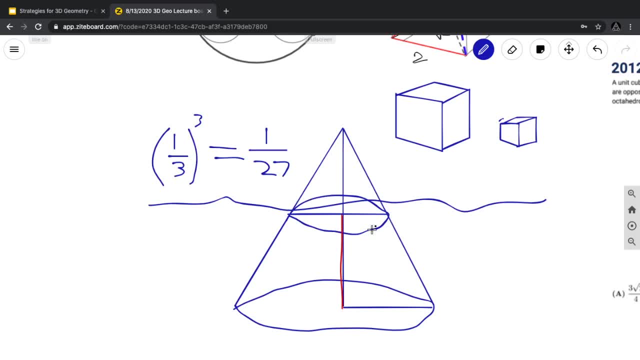 the smaller cone is like, in a way, similar to the larger cone. you can also just look at their side length ratios, Because 1 eighth is equal to 1 half squared. that is our most important observation. Let me quickly clear this junk out. 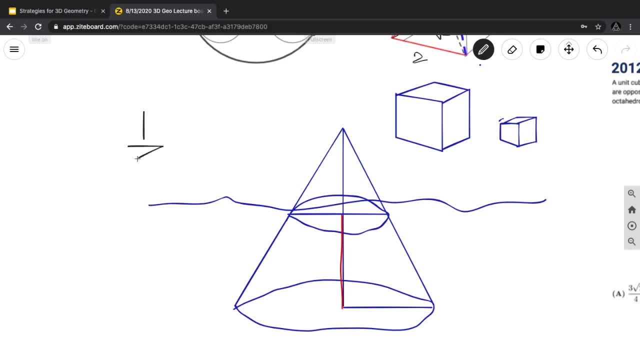 Alright, so we observe 1 eighth. still using the line tool, we observe 1 eighth is just equal to 1 half cubed. So what this means is that the side lengths are actually in 1 half proportion. so this would be 1 half of that. 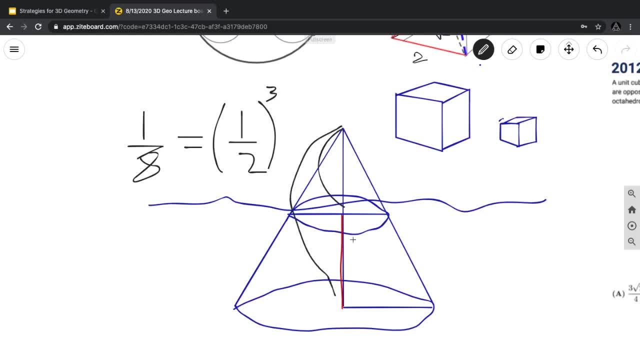 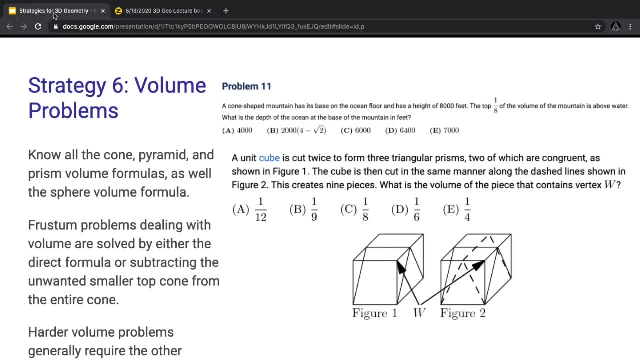 and that is our crux move. Basically, the height is 8,000, and because we split this evenly, due to the side length ratio, the bottom height would be 4,000.. That gives us our answer of 8.. Now the second problem. we'll go over it slightly faster. 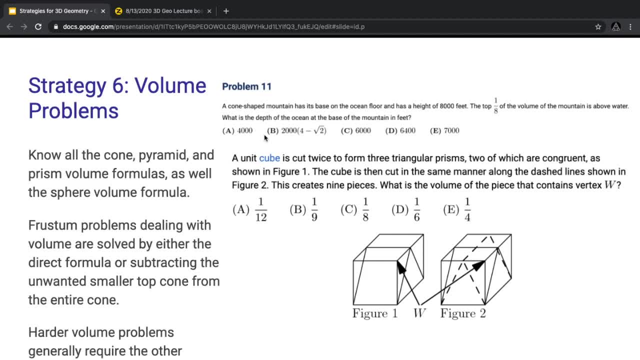 It says: a unit cube is cut twice to form 3 triangular prisms, 2 of which are congruent as shown in Figure 1.. The cube is then cut in the same manner along the dashed line shown in Figure 2.. This creates 9 pieces. what is the volume of the piece that contains vertex W? 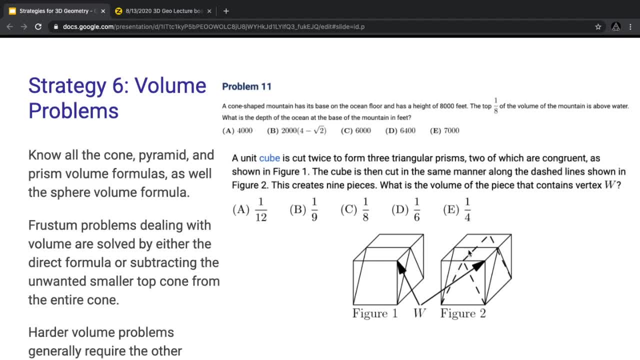 Now, basically, this entire problem boils down to observing that the top face is split into 4 equal sections and the tetrahedron that contains W has a base area of 1- fourth, because that is 1 fourth of 1.. 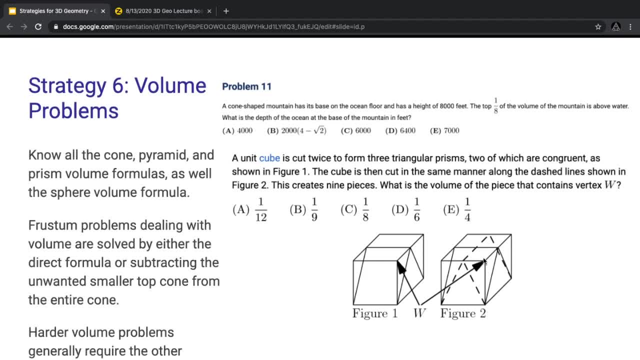 Now to find the height, we observe it's just equal to 1, because it's the side length of the unit cube. so 1 fourth times 1, divided by 3, gives us 1 over 12.. Yeah, sorry, I've been going a little fast for that one. 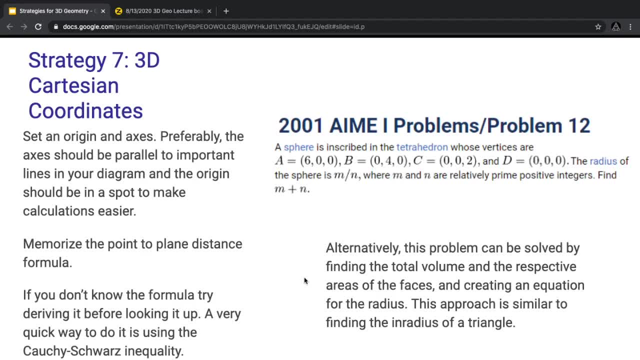 but I just want to move on to the better problems at the end. Alright, so strategy 7. It's about 3D Cartesian coordinates. The best like strategy for this is to identify your origin and axes. Preferably, the origin should be parallel to important lines in your diagram. 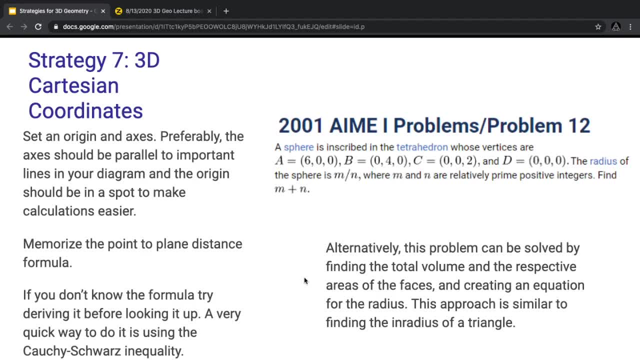 and the origin should be in a spot to make calculations easier. So if you consider the problem on the right, we already see that it gives us an origin which is D, 0,, 0, 0, and the axes are equivalent to A, B and C. basically, 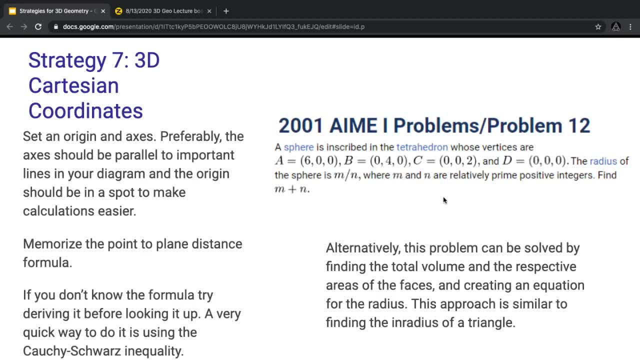 so that makes it slightly easier for us. Now, another good idea is to memorize the point-to-plane distance formula. So what this means is you want to memorize the formula that gives you the distance between a Cartesian point and a plane. 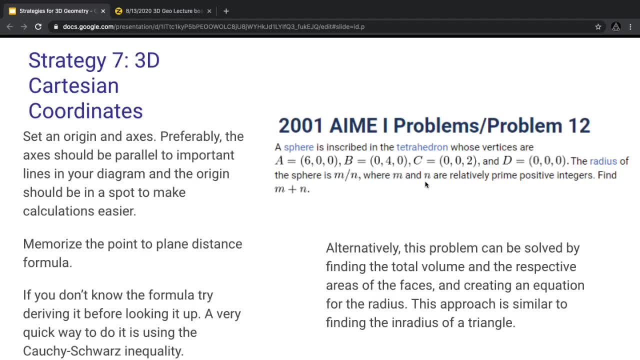 Now, if you don't know the formula, the best way to do it would be to use the Cauchy-Schwarz inequality to prove it. However, you could also look it up. if you're sort of lazy Now, this problem can also be solved using a method. 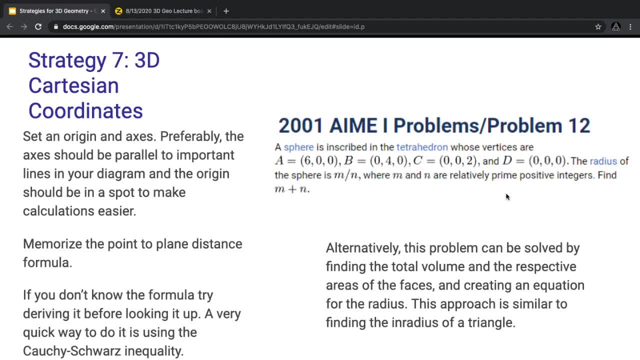 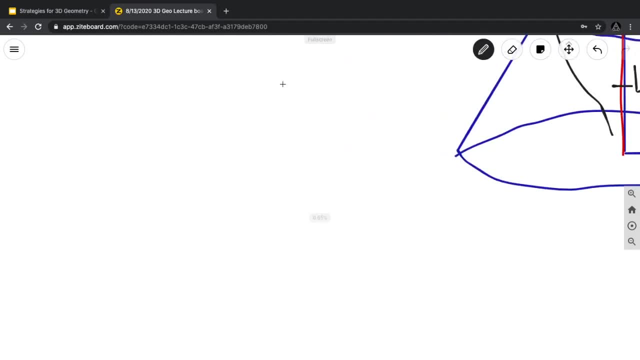 that's similar to finding the in-radius of a triangle, So I'll illustrate what this means in the whiteboard If you're familiar with finding the in-radius of a triangle without a formula. basically, the entire idea revolves around the fact that you can split this triangle into three other triangles. 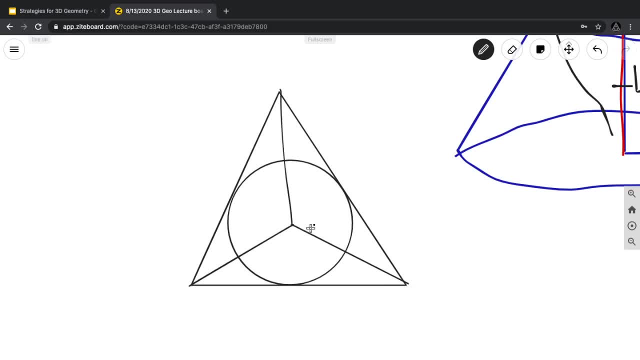 and each of these three triangles has a height of the radius. Just observe when you draw this. So, if you know, tangent lines are always perpendicular to the radii. this is very, very important Geometric fact. So, with this in mind, if we know all the side lengths, 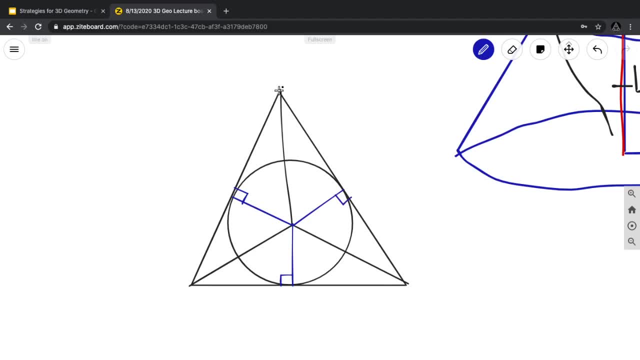 and we know the area. we can find the radius by basically multiplying the side lengths by the radius divided by 2, then setting all that equal to the final area. Now that gives us our in-radius. However, how do we apply this to the 3D problem? 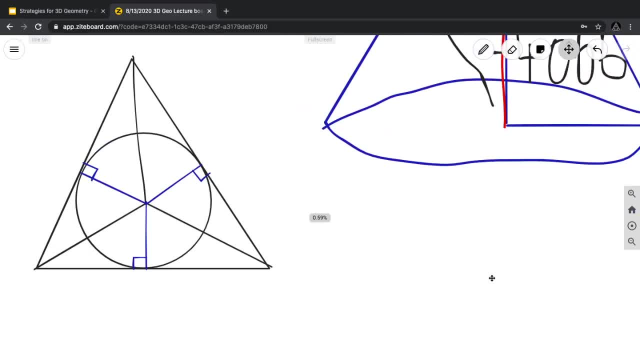 So we're basically going backwards Instead of going from 3D to 2D. we're going from 2D to 3D. So with a tetrahedron instead of finding the in-radius of a circle, 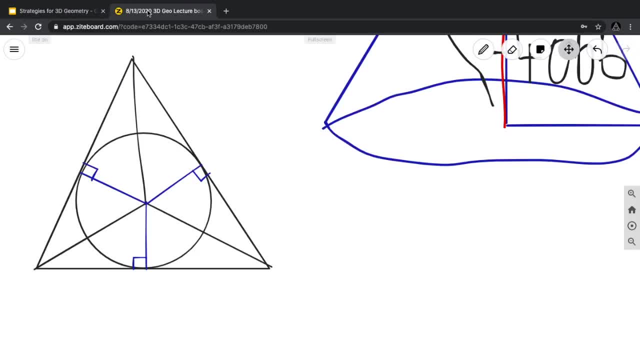 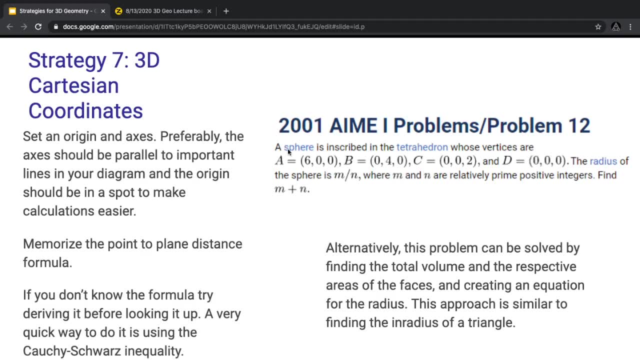 you're finding the radius of a sphere, And it's in the same fashion. We know the entire volume because it gives it to us through the points, and what we need to find are all the areas of the faces. After we find that we can do the same exact method. 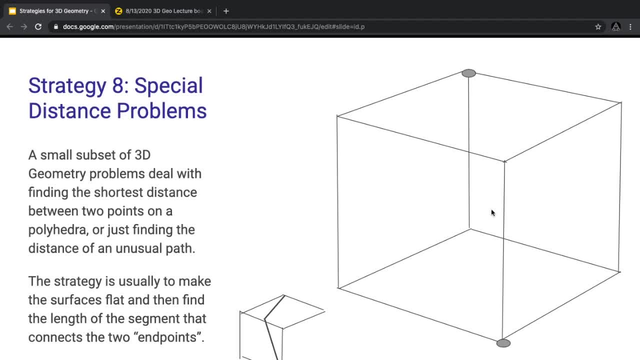 So moving on to Strategy 8.. Now Strategy 8 deals with special distance problems. So a small subset of 3D geoproblems deal with finding the shortest distance between two points on a polyhedra or just finding the distance of an unusual path. 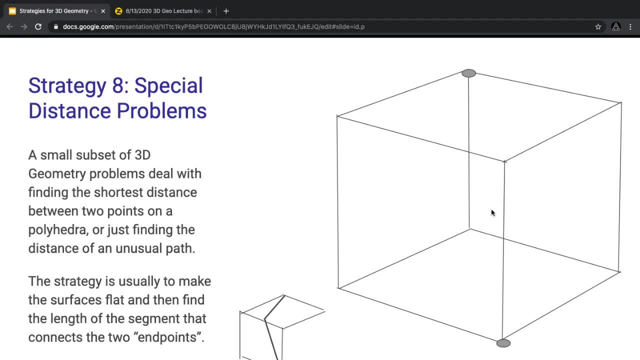 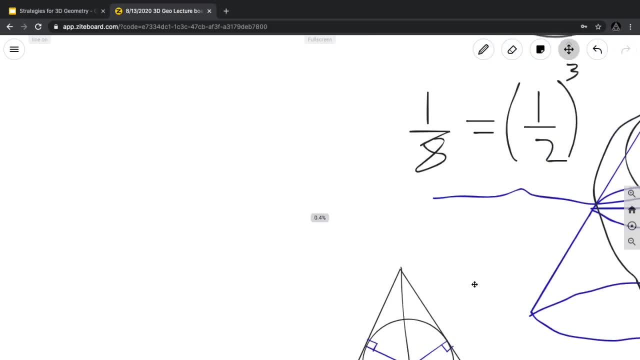 So the strategy here is usually to make the surfaces flat and then find the length of the segment that connects the two endpoints. So this entire idea revolves around the fact, if you're familiar, basically the distance between two points, that shortest distance. 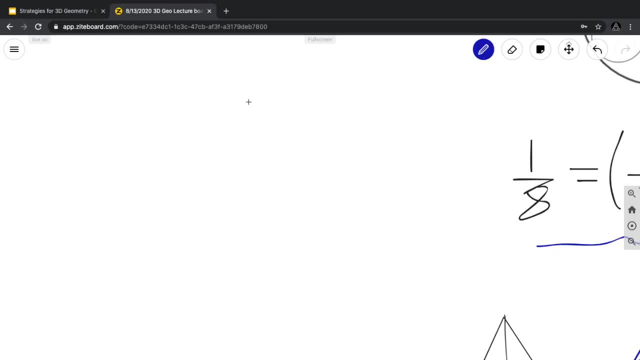 is going always to be the straight line. So we can prove this in a very simple way. Just consider two points. Oops, I deleted the text function, Sorry about that. So if we consider two points and let's just claim that the shortest distance would be the straight line connecting them, 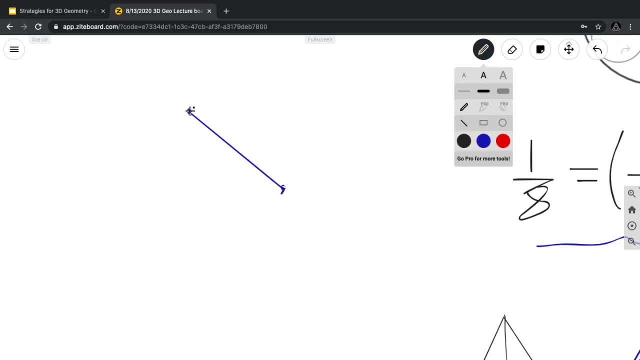 Now how do we prove this right? So let's just consider any other path. So first let it just be like this: So, which means there's a certain angle there. So basically by the triangle: inequality. 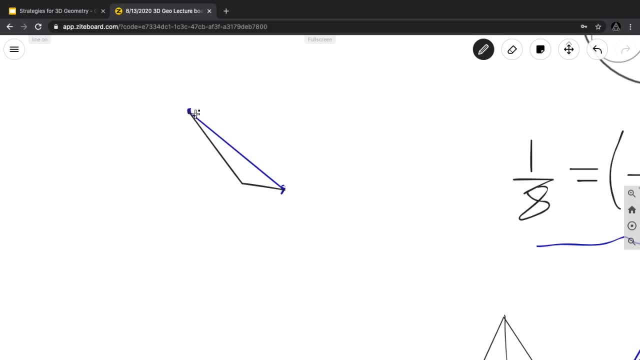 we see that the two black sides added up is greater than the blue side. Therefore, the blue side is shorter. I can apply this to curved surfaces as well as more sides. That would just be more triangle inequality, or probably calculus, if you really want to prove it. 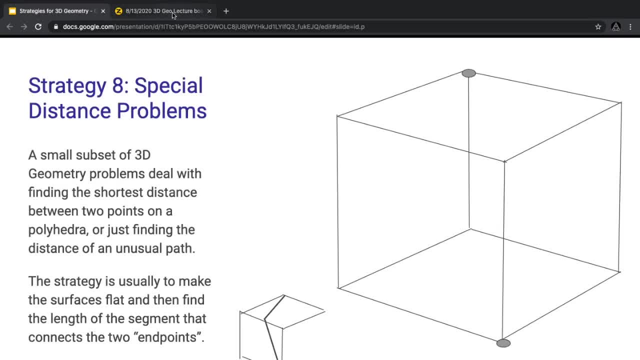 Now, this is just a pretty intuitive thing. So, moving back to the problem here, Basically, let's say we want to find the shortest distance between these two gray ellipses, And it's given that we have to travel on the surface of the cube. 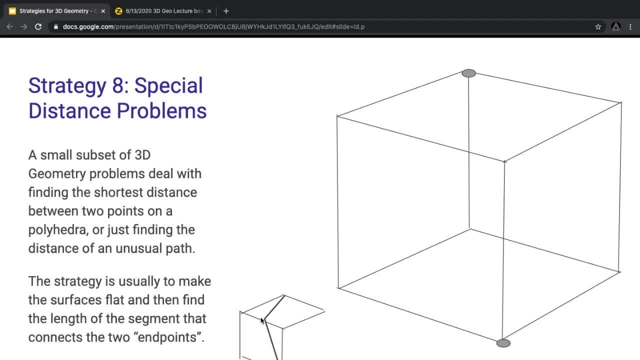 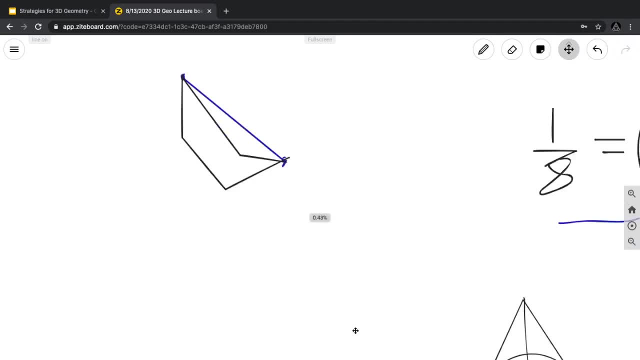 So if you look on the left bottom, this little diagram, that basically shows an illustration of what we're trying to aim for. Okay, so I'll go back to the whiteboard. The strategy is very intuitive actually. So what you want to do, let's just illustrate this cube. 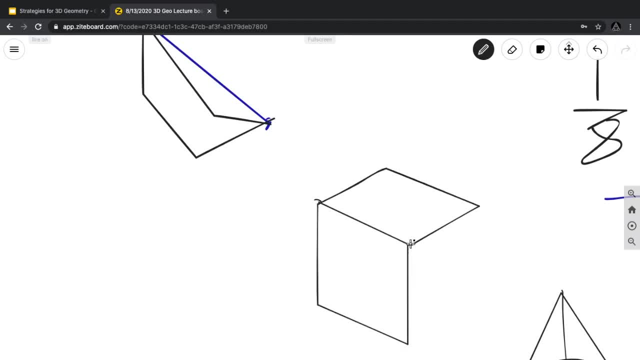 So here are the two sides And we want to traverse the surface of the cube from the top corner to this bottom corner And we have to travel only on the surface of the cube. Now to solve this, what you do, is you actually like? 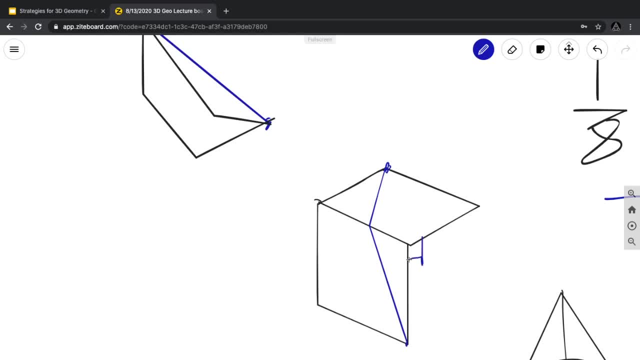 instead of keeping this at 90 degrees, you actually want to like bend it flat, Like imagine pushing this onto a table And what happens is you have this like: oh, that was bad line. You have this like domino-like setup. 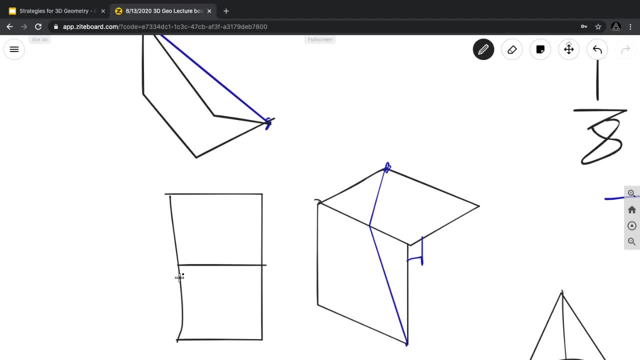 So after you push it flat on the table, you get this setup Alright. so we have this top point up here Looks like this, and we have a bottom point down here. So if we want to find the shortest distance, then this is pretty clear. 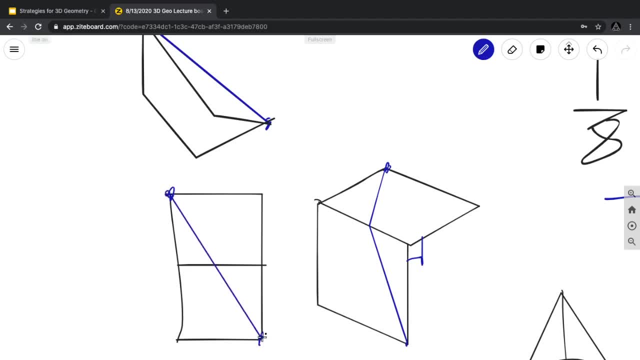 We just apply that triangle inequality I was mentioning to prove that this is the shortest distance between the two points And reflect it. This is like bad drawing, But of course these two segments would be equal. if we're considering this is a unit cube. 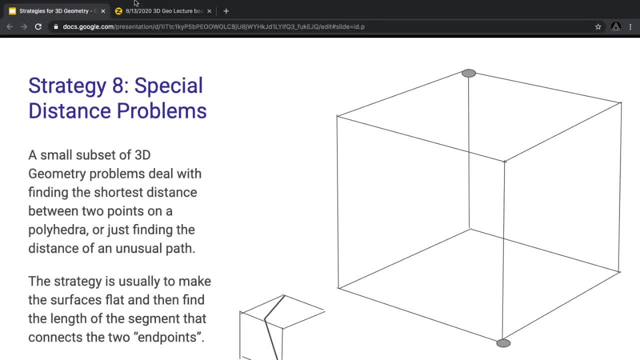 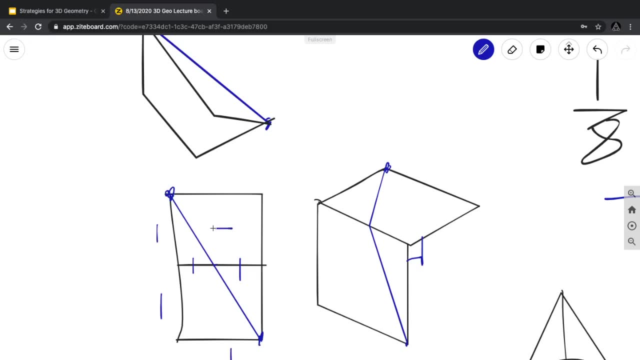 Now, that's basically how you solve this problem, And if it tells you to find the length, this would just be 1,, 1, and 1.. And then, by Pythagorean, this would be root 5. Okay, 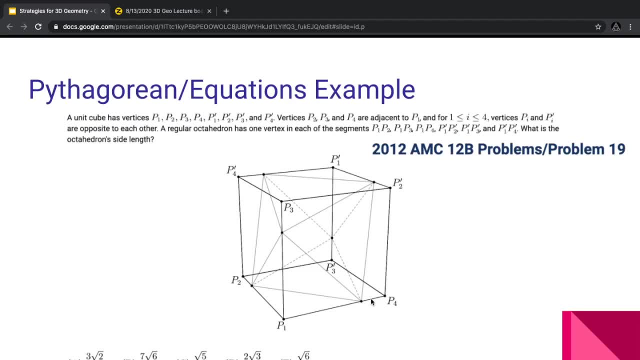 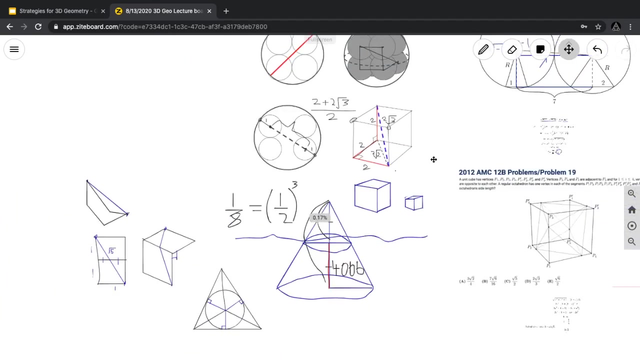 Moving on from strategy 8.. Let's consider this Pythagorean equations example. Just give me a second to drink some more water, Alright, Alright. so it reads: The unit cube has vertices P1, P2, P3, P4.. 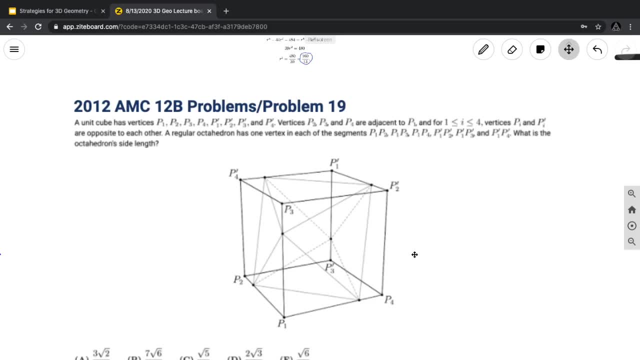 P1', P2' P3' and P4' Vertices. P2, P3, and P4 are adjacent to P1.. And for i, greater than or equal to 1,, less than or equal to 4, vertices Pi and Pi' are opposite to each other. 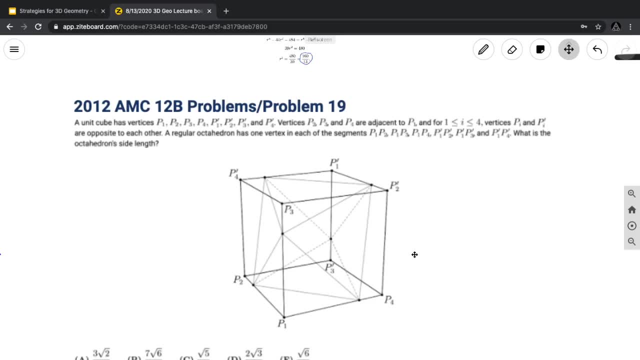 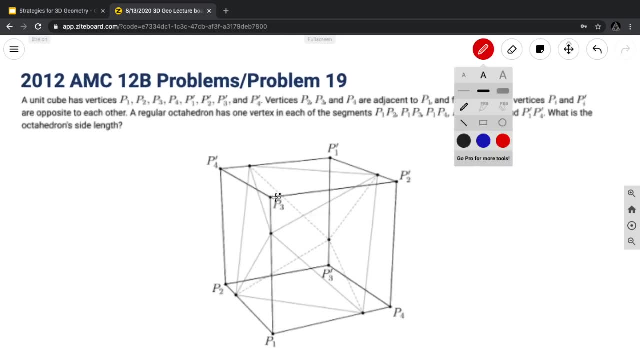 A regular octahedron has one vertex in each of the segments of the cube. What is the octahedron side length? Firstly, observe by symmetry that- sorry, give me a second- that this length would be equal to this length. 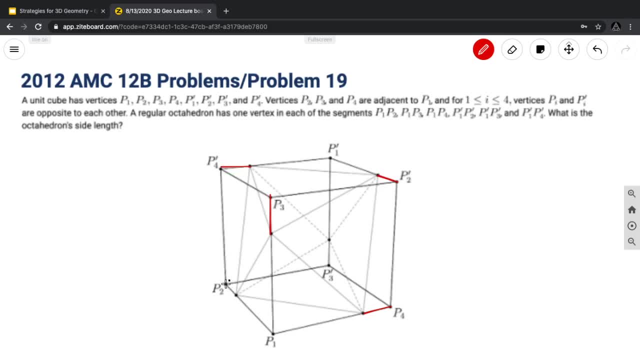 equal to this one, equal to this one and this one and finally this one. And that's because of the nature of the octahedron. Every side length of the octahedron is equal, which means like this is equal to this. 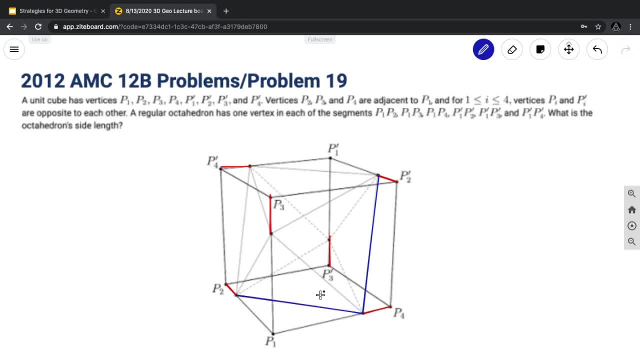 which is equal to this guy. Now we want to find the octahedron side length correct. So the entire idea is based on Pythagorean, of course, given by the name. So to find, let's just try like finding this the first one. 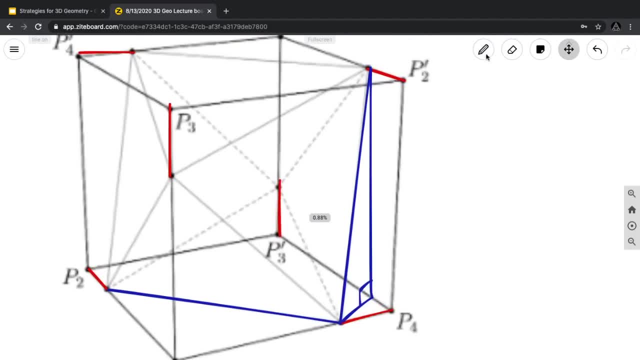 So the entire strategy is right here. It's actually not very hard to observe this. What we want to do is set us a length of x for like this part, So we have a variable now and then we have 1.. 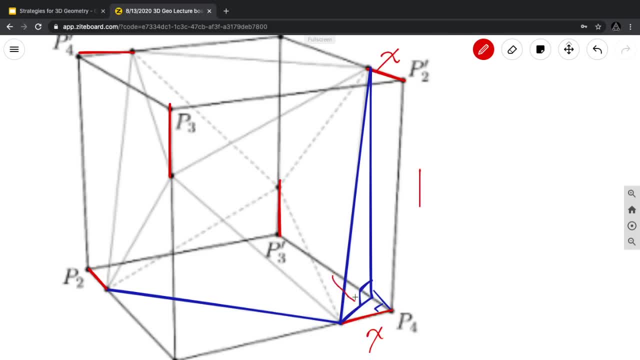 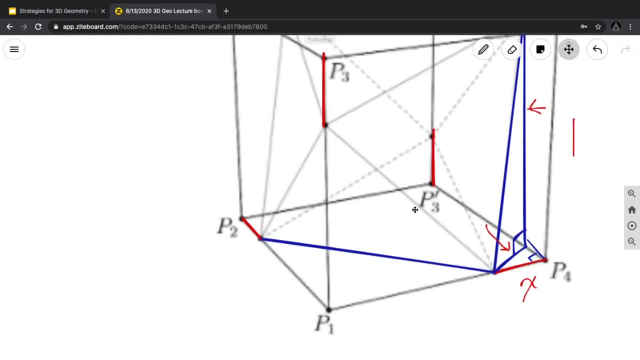 And by Pythagorean we see that we have an x root 2 here, and then we also have 1 here, And then we use Pythagorean one more time, And on the other side, what you want to do is just say this is 1 minus x. 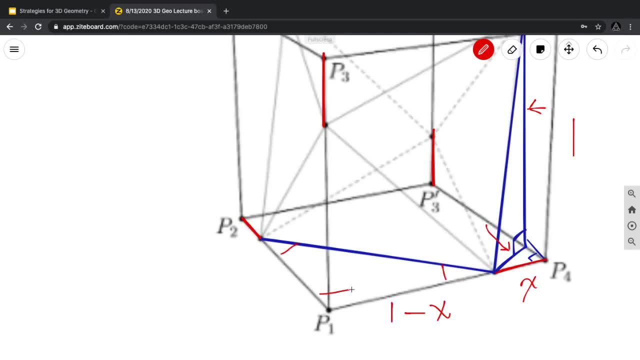 and we observe this is a 45.5.. 45, 90 triangle. So then this would just be equal to root 2 times 1 minus x. So I prepared the rest of the calculations just to save some time. 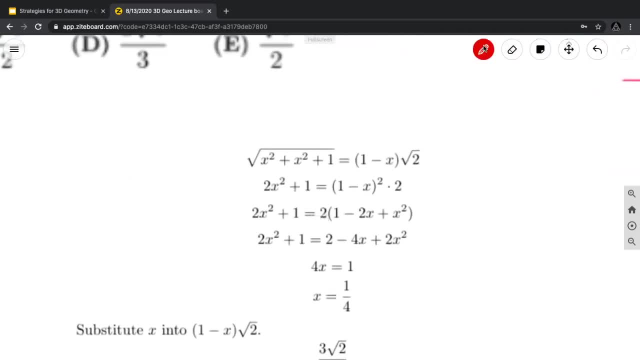 They're right here. So basically we have those two lengths and then we solve for x. And remember, x is just a small side length. What you actually want to calculate is the length of the octahedron, And, of course, all you have to do is substitute x back into the original equation. 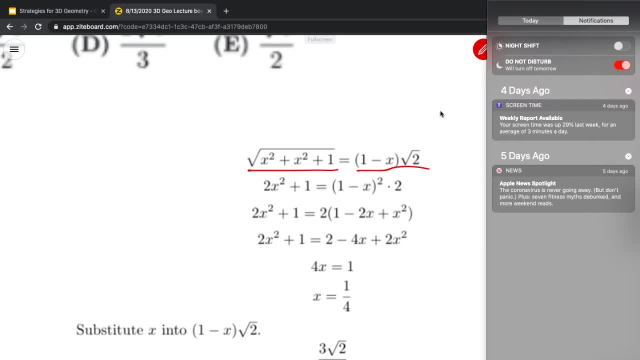 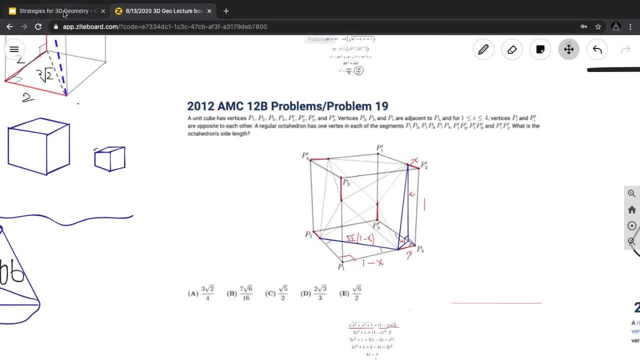 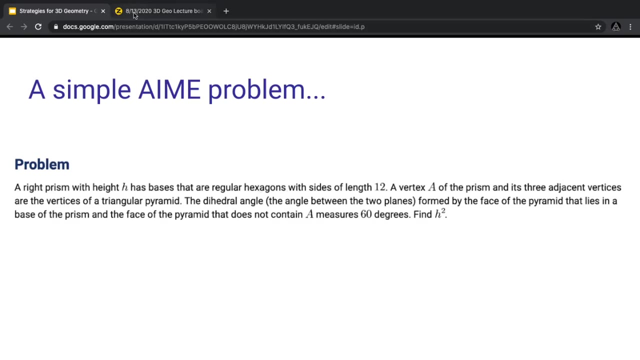 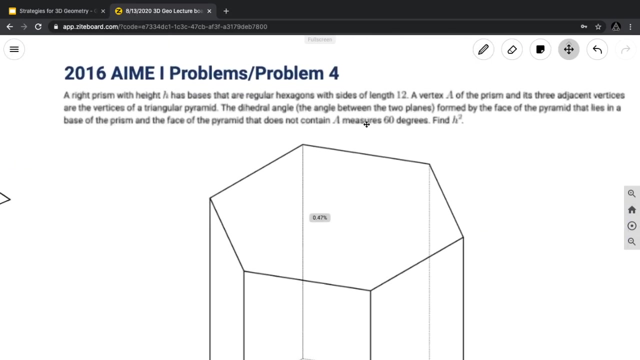 and this gives us 3 root 2 divided by 4.. Okay, So that would be answer choice A. Alright, So my next topic is an Asimple-Amy problem. This is the 2016 Amy-I problem 4.. 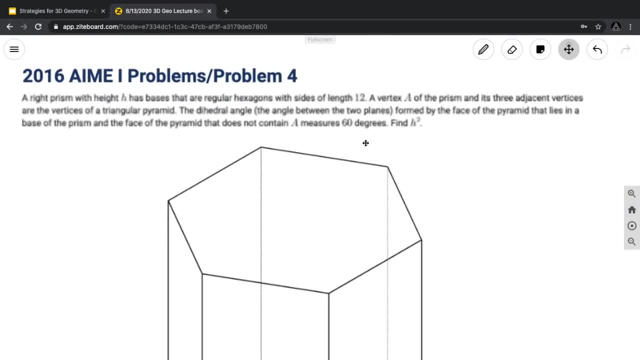 It reads: A right prism with height h has bases that are regular hexagons with sides of length 12.. A vertex A of the prism and its three adjacent vertices are the vertices of a triangular pyramid, The dihedral angle or the angle between the two planes. 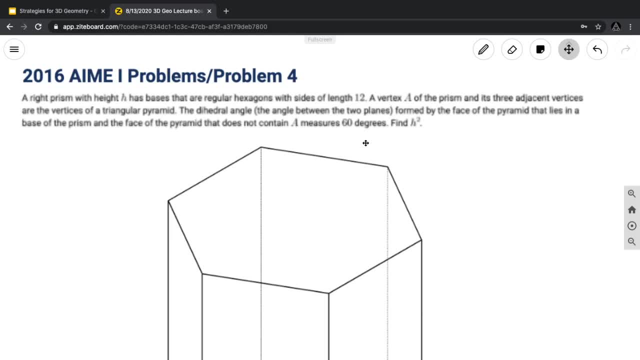 that is formed by the face of the pyramid, that lies in a base of the prism, In the face of the pyramid that does not contain A. this angle measures 60 degrees. Please find h squared Now. I'll give you all some time. 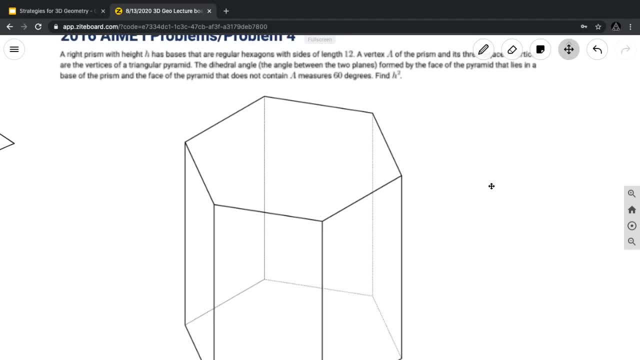 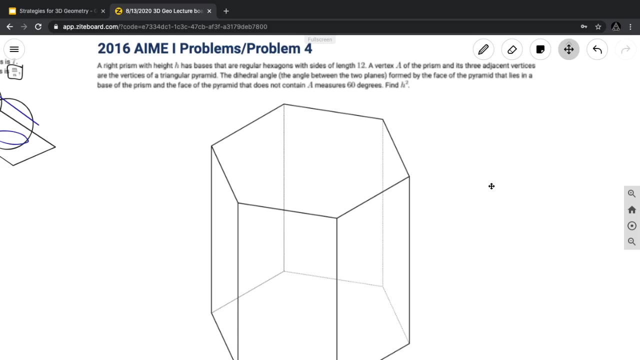 to think about this problem, Maybe 2 to 3 minutes, And if you guys have any ideas, just put it in the chat, please. Alright, Oh, Sorry about that, Shh. Oh, my goodness, I'm sorry. I'm sorry. 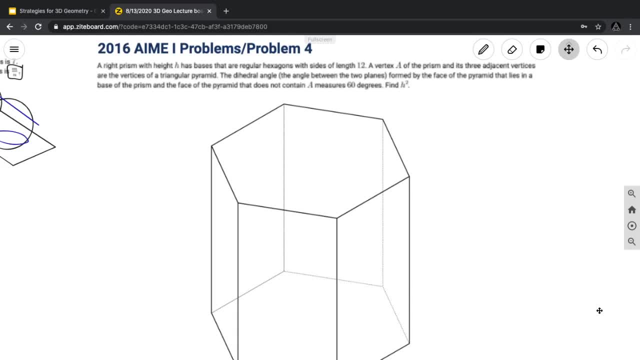 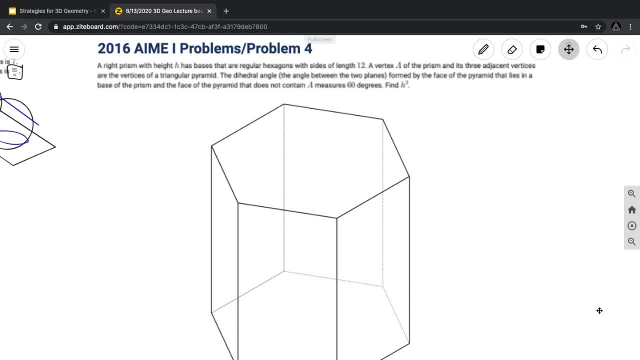 And it's totally fine. if you don't have any ideas, I think we should stop and start solving now. Alright, I'll walk everyone through it. So basically, the entire idea is that there's two faces we're considering on a triangular. 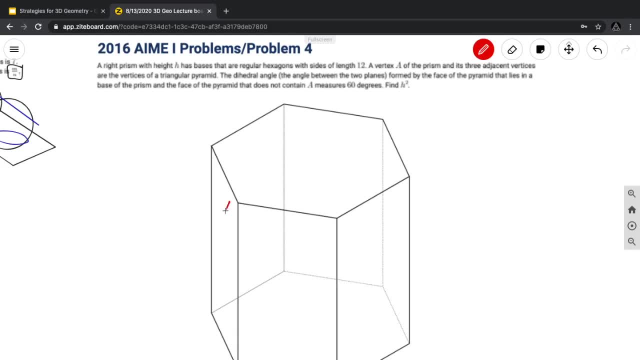 pyramid. So the first thing we want to consider is that this would be A. Let's just call that vertex A, And then we'll call the other one. we won't call them anything, but we'll just consider the other vertices of the triangular pyramid. 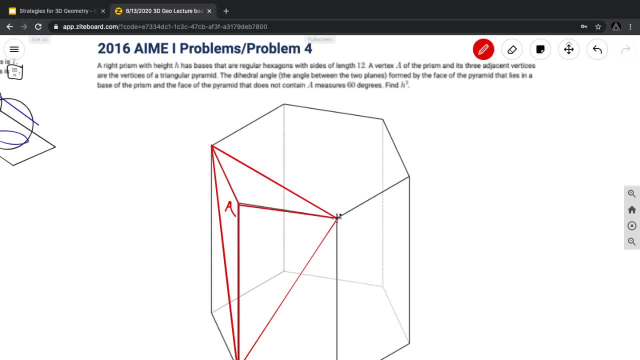 Now this is the triangular pyramid they're referencing in the problem and what we want to do is find the angle between. so this is going to get a little messy. we're going to try to find the angle between this top face and the back triangular face. 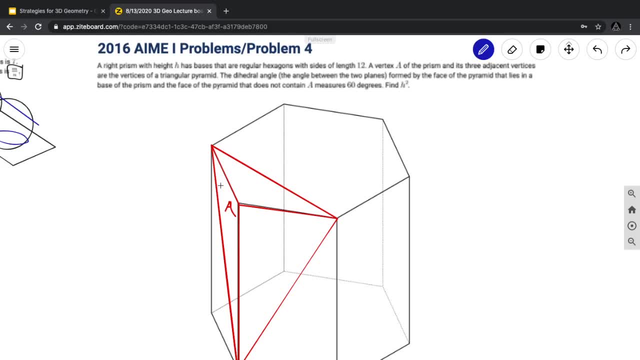 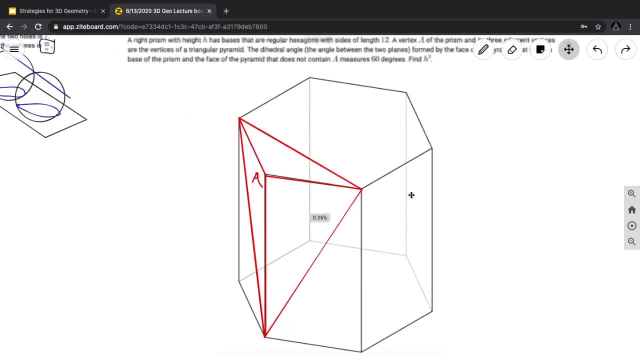 Alright, so how do we do this? Okay, So basically, what we want to do is figure out how to represent the dihedral angle, Like, how do we get this angle into our diagram so we can actually find it? It's actually not too hard. don't overthink it. 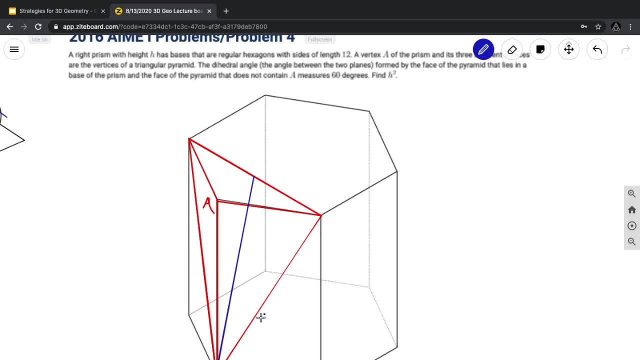 What you want to do is consider a line that lies on the plane, Then we want to connect it with a line that lies on top. But basically, because you have to preserve symmetry here, you have to make sure everything is referencing the same segment. the best way to do this would be to draw the perpendicular. 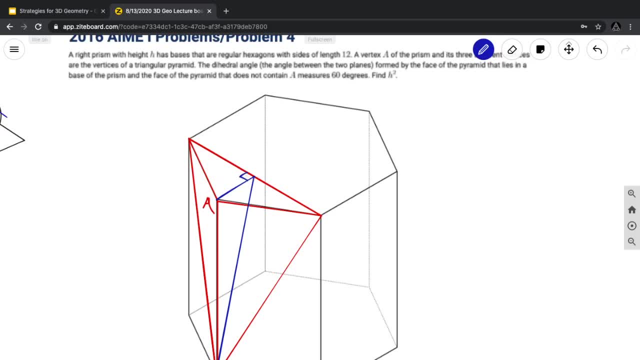 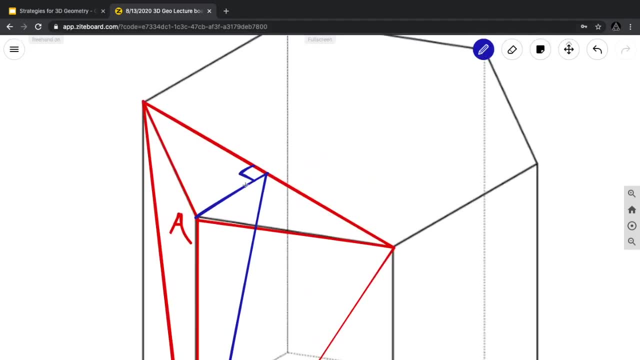 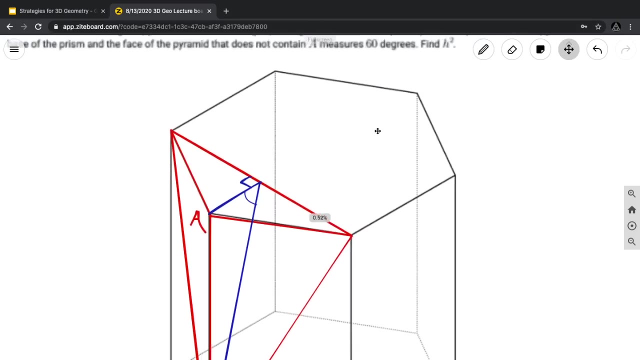 bisector of the top face and then connect it, connect that endpoint with the bottom. So what does this do? This gives us a very unique angle right here. This angle is precisely 60 degrees, given by the problem. Now we observe immediately that, since this is 90 degrees and that this is 60 degrees, 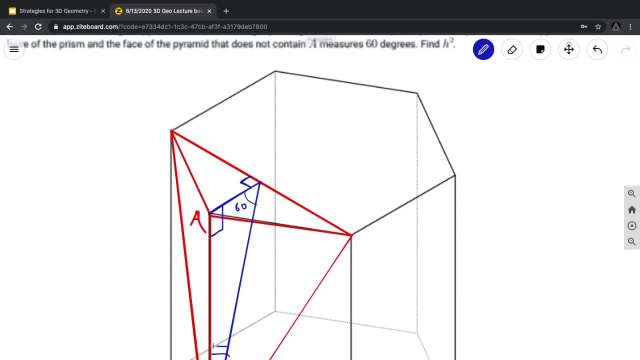 we have a 30-60-90 triangle, which is great because this makes calculations much easier. Now we also observe on the top. So because this is a regular hexagon, we could just draw a similar triangle right here. And if we draw the perpendicular bisector, this is also a 30-60-90 triangle. 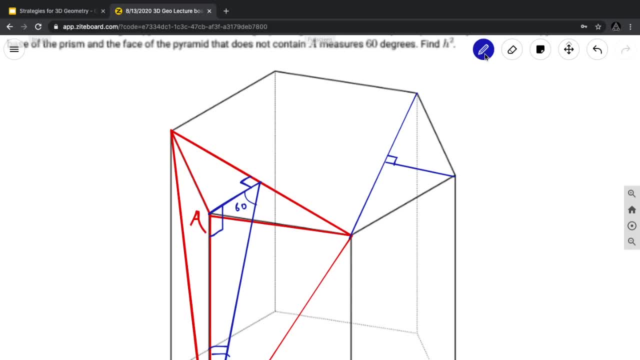 This also creates two 30-60-90 triangles. All right, so if that's true, then we see that we can also utilize the side lengths again. Now, one of my colleagues just mentioned if you all are not able to talk in the chat. 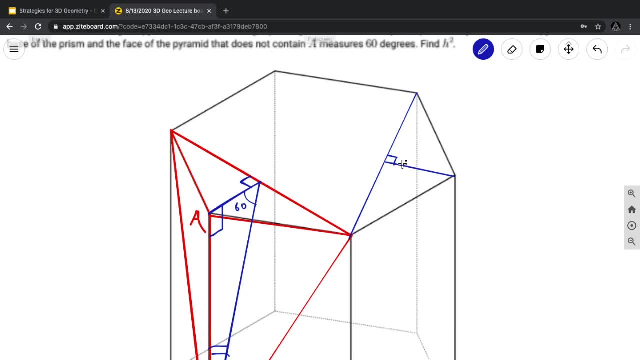 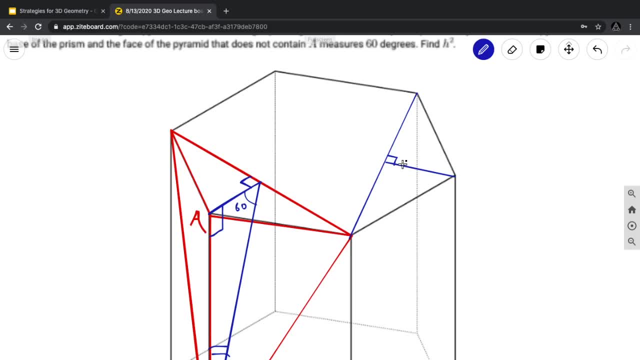 talk if you would like, But of course you don't have to. But if you do make a Twitch account, please just follow us and ring that notification bell. Now back to the problem. If this is a 30-60-90 triangle, we also know that the side length is 12, right. 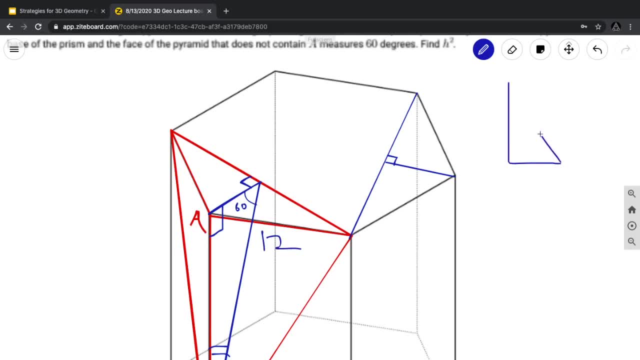 So then, by 30-60-90 ratios of 1,, root 3, and 2,, that means that this length is 6.. Now This is great, because as soon as we have 6,, we can see that we can use our second 30-60-90 triangle. 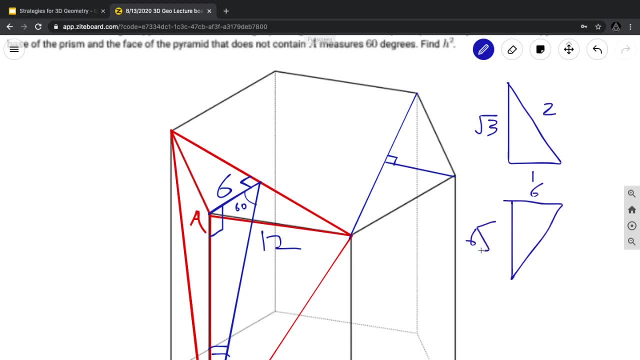 So we have 6.. Therefore, this is 6 root 3 by the 30-60-90 ratios. And finally, our height would be 6 root 3.. And when we square that, we get 36 times 3, which is the same thing as 108.. 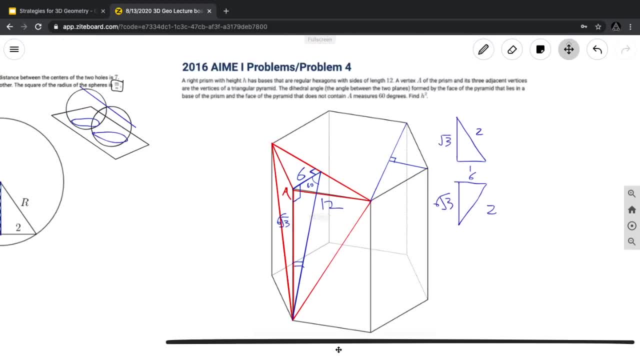 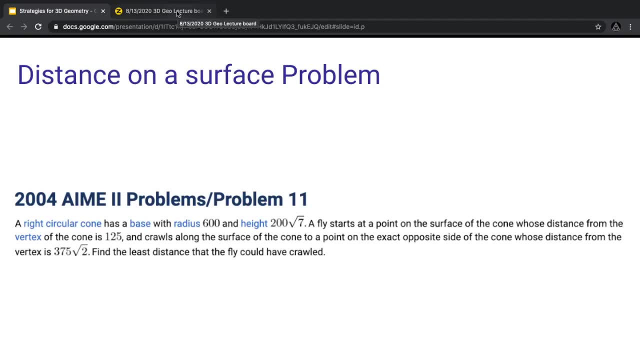 So that is our final answer. Okay, now let's go on to the last problem, And after the problem we'll have Q&A sessions. Unfortunately, not all of you are talking in the chat, so it might be hard to get problems across, but we'll see what happens. 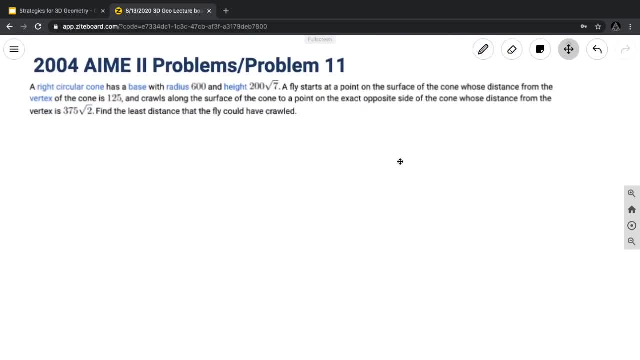 Alright, so our last problem is an Amy II problem, So I'll read it real quick and I'll give you guys maybe a minute to think about it. So the problem reads: A right circular cone has a base of radius 600 and height 200, root 7.. 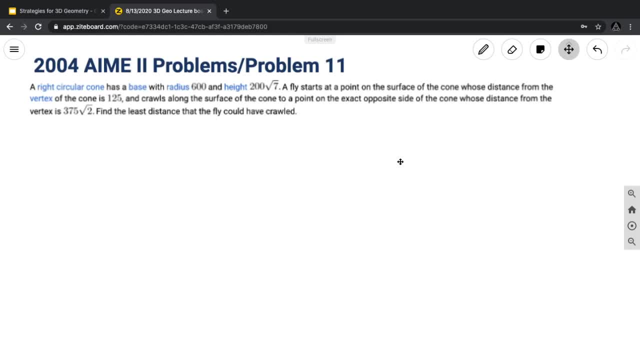 A fly starts at a point on the surface of the cone whose distance from the vertex of the cone is 125, and it crawls along the surface of the cone to a point on the exact opposite side of the cone whose distance from the vertex is 375, root 2.. 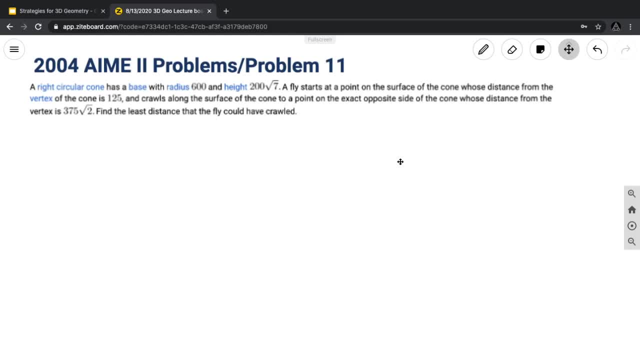 Find the least distance that the fly could have crawled. Just one minute to think about it, Salie. what's your washed line number here? Salie, you have your right, left, right, left, right, left, So right is the. 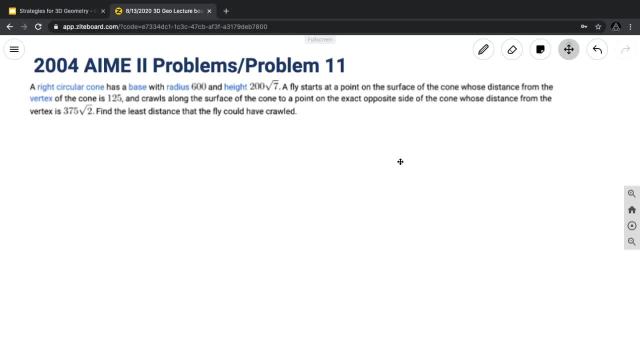 right radiusess of the line that else cut through A têm. Okay, I think we'll just get started with the solution Now. first we have to visualize it right. So this problem gives some quite unusual parameters, but, however, if you just think about it a 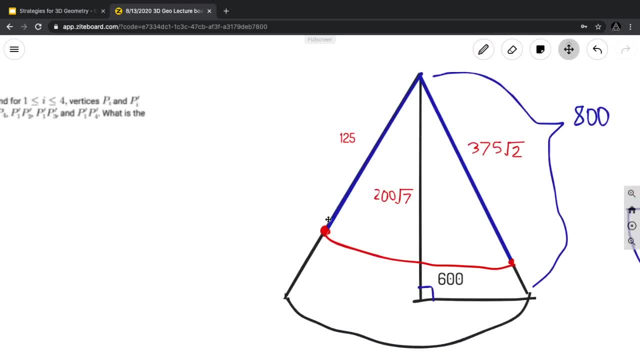 few minutes, you'll be able to figure out that the cone and the diagram looks something like this. So our fly starts right here. So actually this is a quite an interesting fly. it actually decided to walk, So I have no idea what the problem creators were thinking. 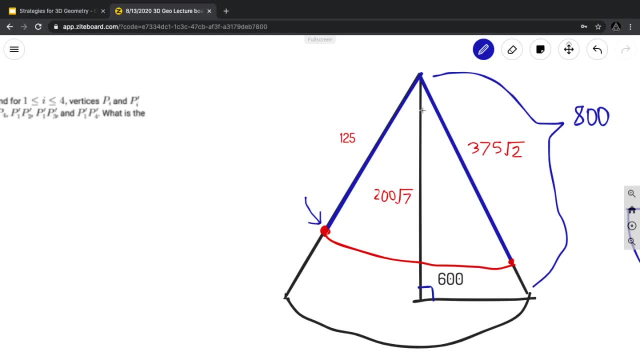 Now, if it starts here and it goes to the opposite side of the cone, that just means that if you just traced its entire journey on like the ground, maybe, for example, it will just be a diameter of the cone. Now, with that out of the way, our first strategy is to realize that it's like the distance. 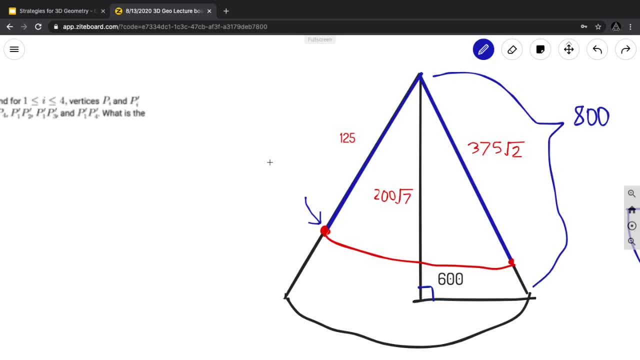 on a surface problem, What we want to do. uh, okay, so someone said, is it 625?? Yeah, that's right. I mean, like you provided an answer without much of a solution, but that is correct. So yeah, now moving on to the actual problem: what we want to what? the entire strategy. 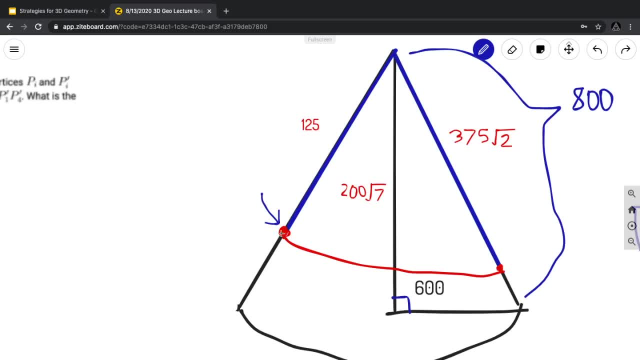 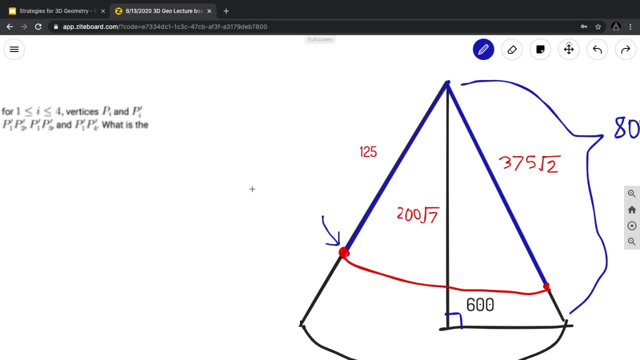 is is to make this cone into a flat surface. Then we connect the two points on it. So, if you remember, the shortest distance between two points on a surface would be a line, and that gives. that would give us our answer. Now for those who are not familiar, if you basically put a cone flat on a surface, what 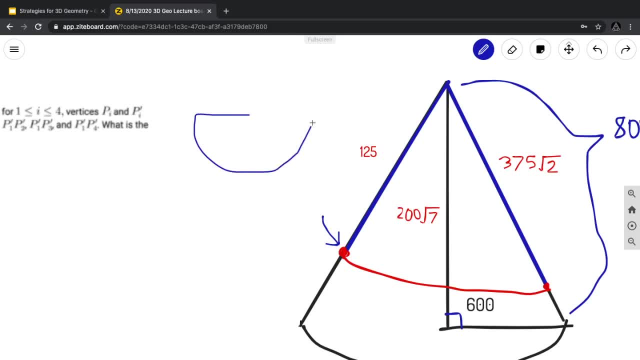 happens is that it might create something that looks like this, Like it looks like a Pac-Man. Basically, uh, it's a circle, but it's missing a sector. And when you tape like let's imagine taping these two ends together, this becomes the. 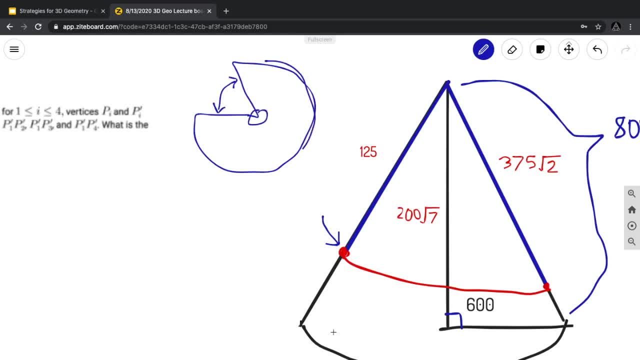 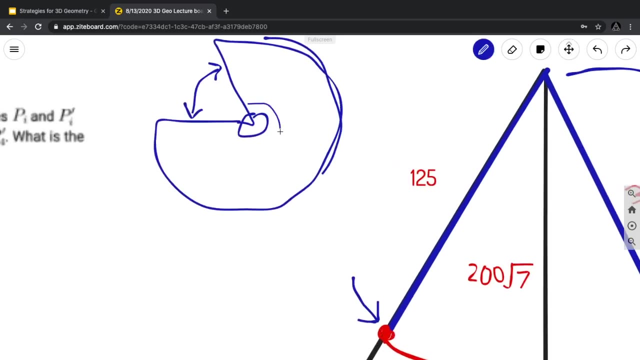 vertex and the outside perimeter- Okay, It becomes this bottom perimeter. So, with that in mind, what we want to do is first figure out what this- uh- outer session looks like. So the two parameters that give us this outer session is one, this central angle, and two. 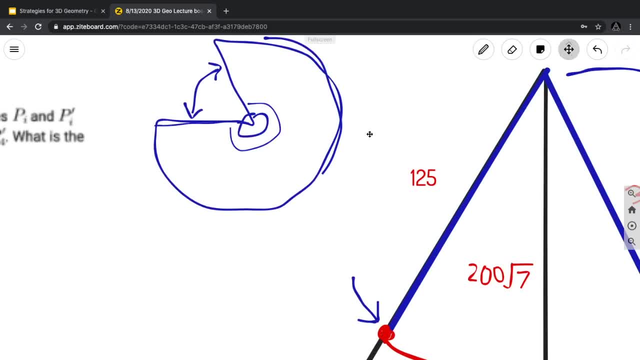 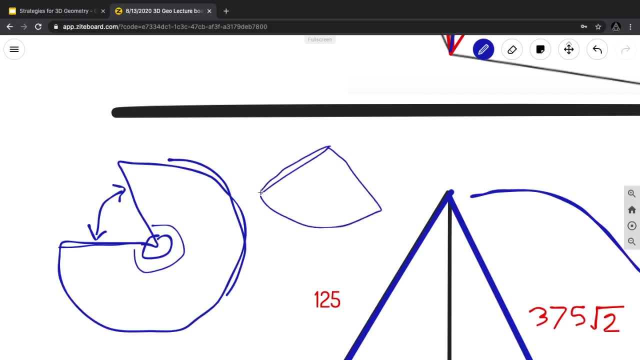 the radius. So first let's deal with the radius. the radius: Uh, if you just observe, by folding these two edges together you create the cone right, And those two edges, of course, would be a slant height. They would be this distance. 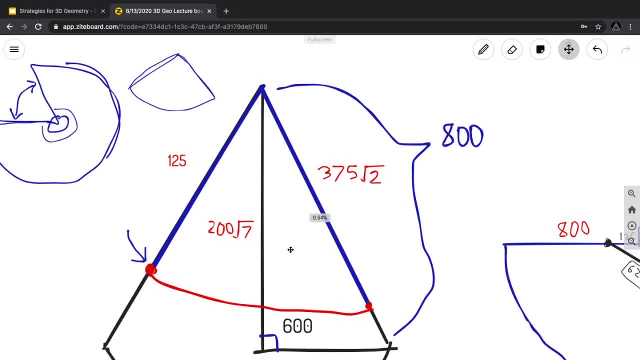 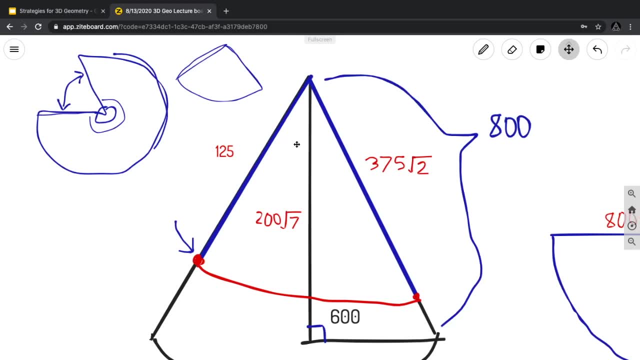 And, of course, by using Pythagorean. I'm saying, of course, a lot. by using Pythagorean, we're given the height and the radius. So we see that the slant height would be 800, and you can verify this, of course, if you. 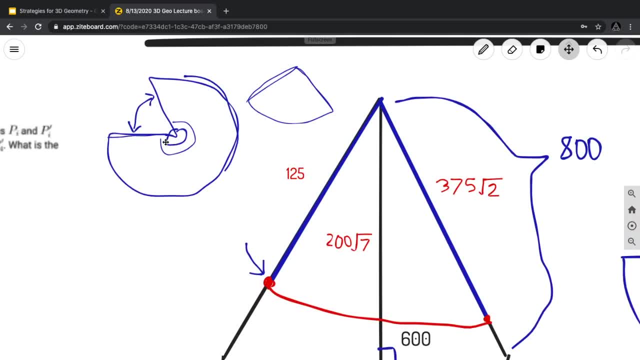 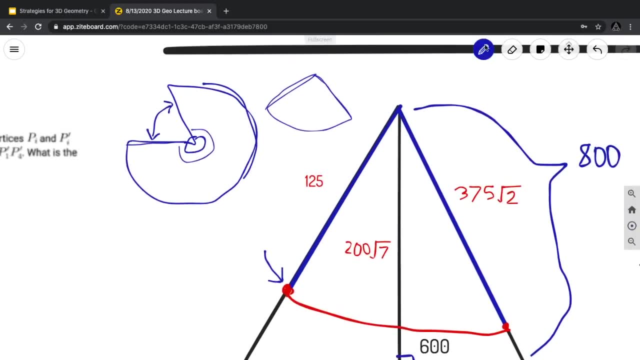 would like. Now we have the radius and we want to find the central angle. So to find the central angle, it's actually quite a neat method. What you want to do is first figure out, so I'll use some different colors. You first want to figure out this length in red, then you want to divide that by the total. 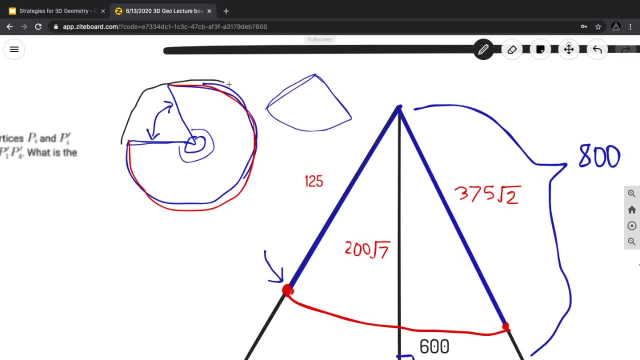 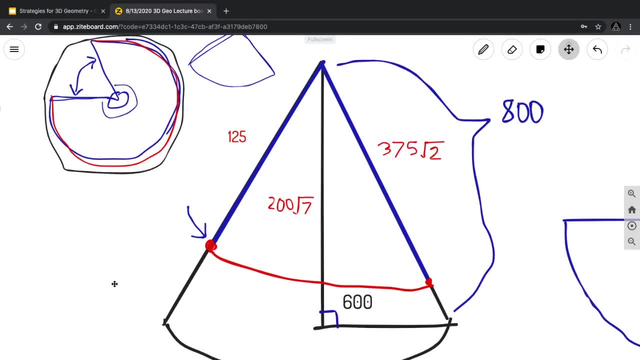 Okay, You want to divide that by the total circle circumference, which is in black, And as soon as you get that, you're going to have a ratio of basically the sector angles. Now, how do we find the red length right? So, once again, that red length is actually interesting. 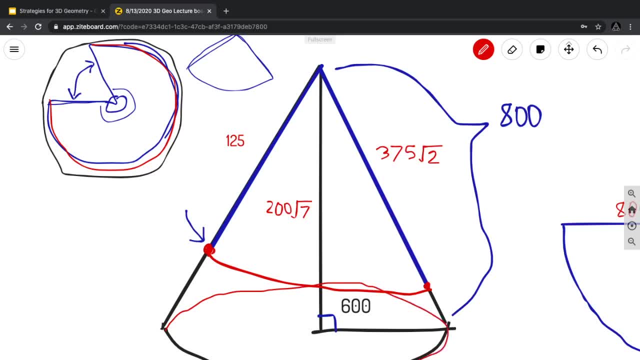 It's just the perimeter of the base of your cone. That's quite interesting. It's not hard to verify. If you just imagine splitting the cone again. most of this should be pretty clear now. to find the base perimeter. Of course, That would just be 2 pi r and we have 1,200 pi. 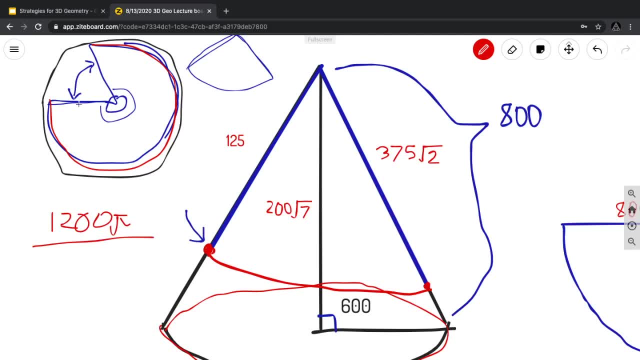 Now we want to divide that by the total circumference. What is the total circumference? Well, recall that the radius is 800.. Excuse my poor handwriting. Therefore, the total circumference would be 1,600 pi. Now, this simplifies to 3 over 4, which is very, very nice. 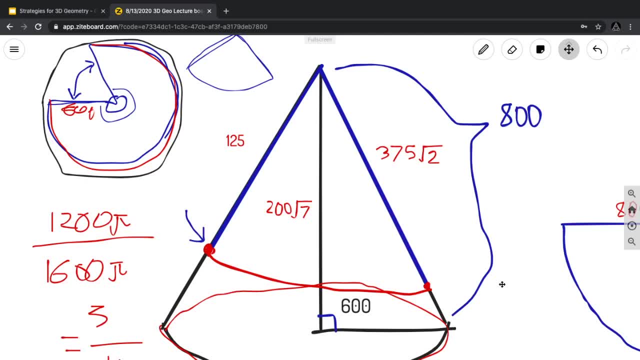 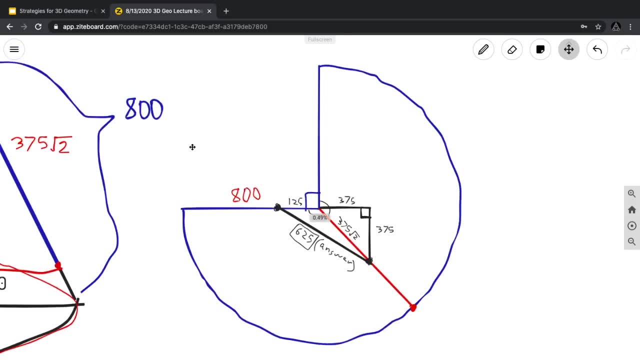 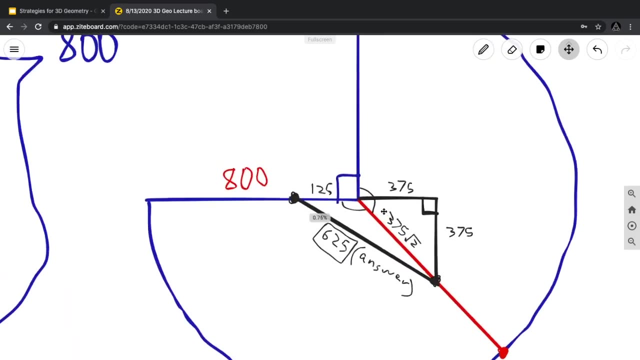 3 over 4 just means that we're taking out 90 degrees, So we have 270 degrees as the central angle. So let's move over to our right diagram. This is going to be the second part of our solution, So first we should transfer all our side lengths over. 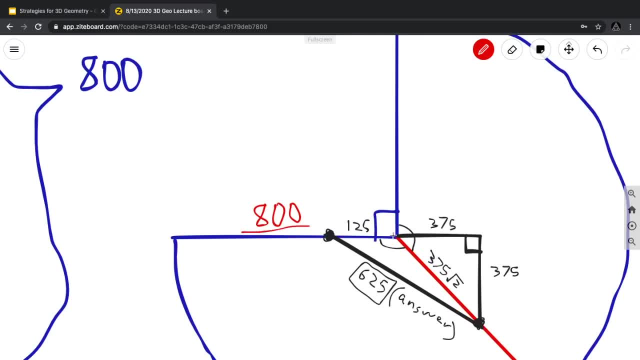 We basically have a radius of 800, which is right here- And we have that starting point with a distance of 125 from the vertex, And then we also have that opposite point on the opposite side of the cone, which is right here. 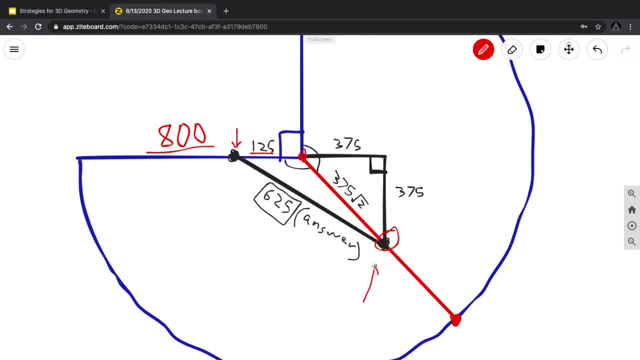 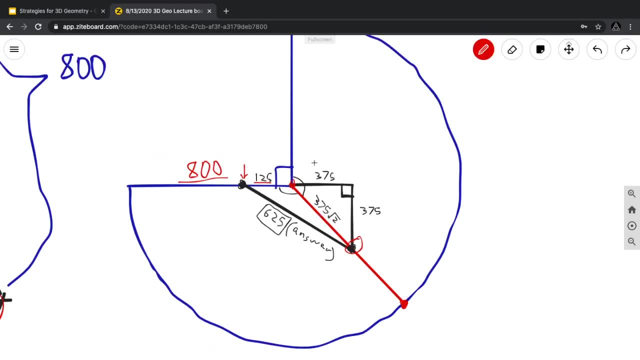 Now you might be wondering: why is the opposite point like weirdly positioned? Shouldn't it be like over here, maybe? No, That's actually incorrect because, remember, this is like the folded out version of the cone. So imagine if we said: because you first have to recall that these two edges are the same. 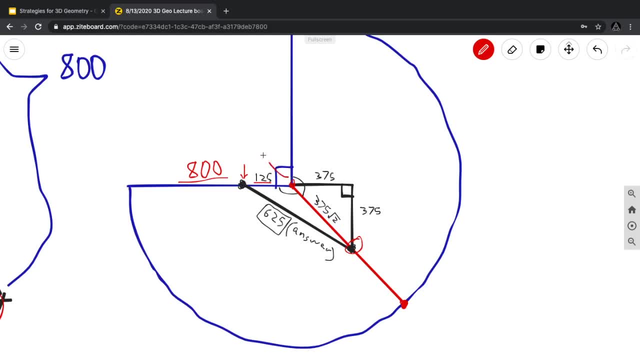 thing when you fold them together. So when you fold them together they might end up like around here, And of course the opposite side of this would be over here, So that by symmetry we also know that the central two angles are the same. 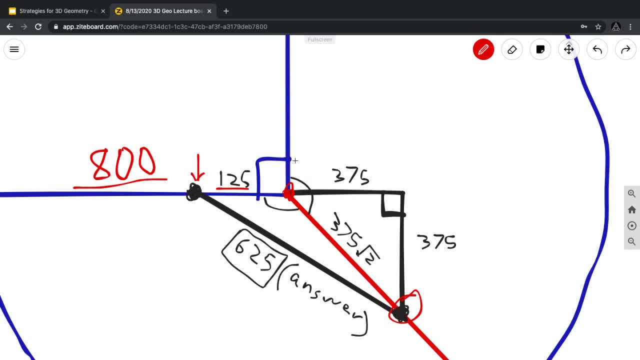 And because the total central angle was 200 pi, we also know that the central two angles are the same. And because the total central angle was 200 pi, we also know that the central two angles are the same. But we can also see that. we can also see that if we make this angle with the x-axis, we 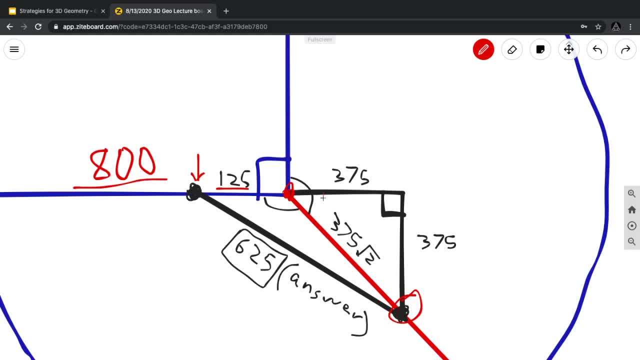 can also see that if we make this angle with the x-axis, we also see that this angle is 175.. And if we extend this angle to 470, this angle is 135.. And because this is 90 degrees, this is 45 degrees. 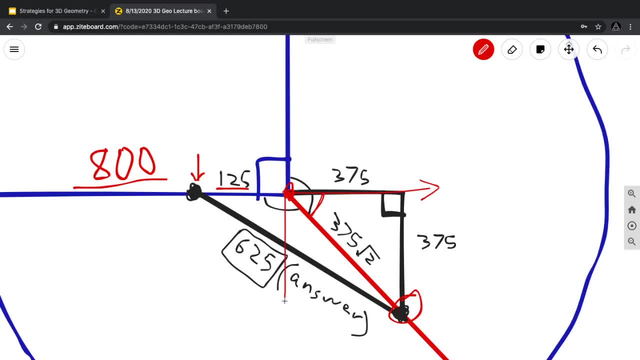 And, of course, if we extend this outwards by symmetry, we could also extend it this way, and this creates a square. Therefore, this is 90 degrees. when we draw this height down, and we have a right isosceles triangle. All right, this is very, very good. 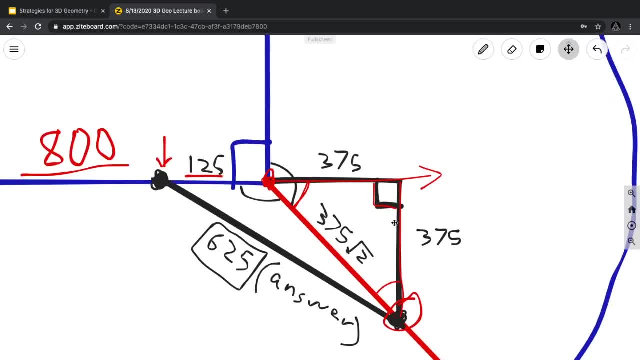 The reason why is because we have all these side-length ratios in a right isosceles triangle And of course the problem makers were kind of lazy here, So they directly gave us a, a very unique number, 375 root 2. but if you recall the right isosceles triangle side ratios, they are. 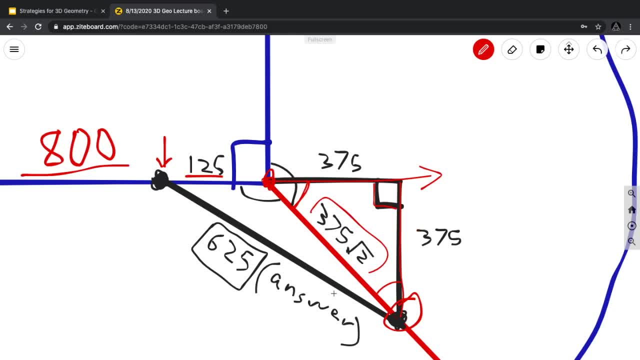 in the ratio of 1: 1 root 2. so, of course, all you have to do is divide by root 2, which gives us 375 and 375. here now we're on the home stretch. basically, all we need to do is create the right. 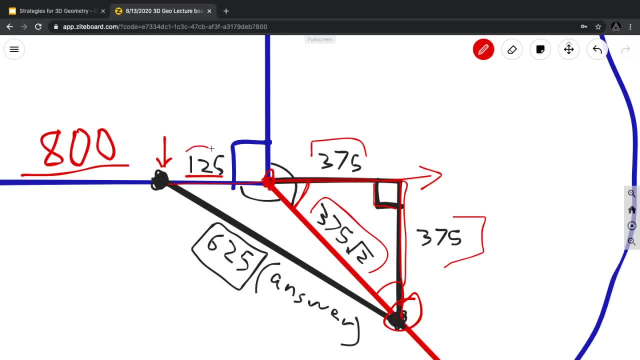 triangle here and use pythagorean, so this is given to be 125, and then 125 plus 375 is equal to 500, and then we also have 375 over here. so 500 squared plus 375 squared should equal 625 squared, and 625, because it's a straight line. this is the shortest distance between the two points. 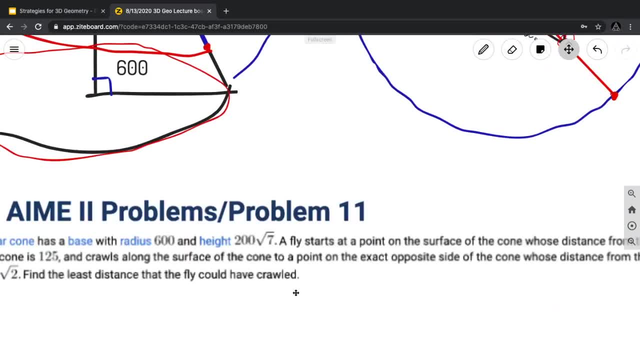 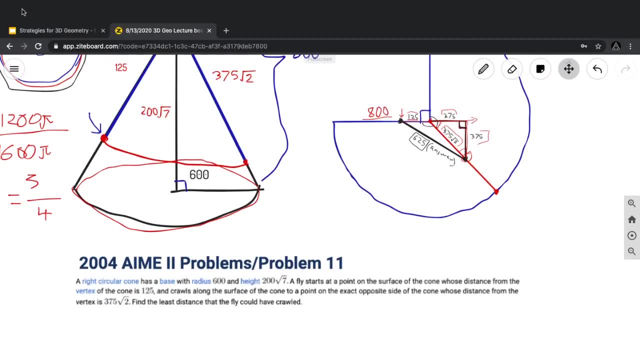 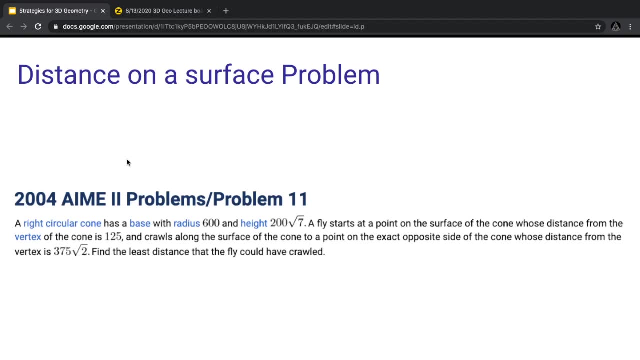 so our answer would actually be 625 and derrick, 343 in the chat is correct. all right, so unfortunately, that concludes our lesson for today. first, i'd like to point out we also have a discord channel. i think one of my colleagues could put that in the chat. i'll just do it because i don't see one yet. 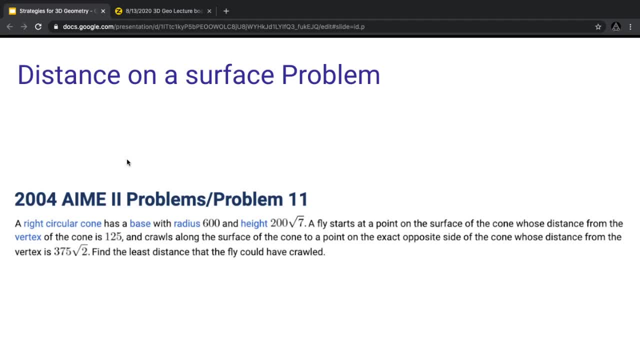 all right, just give me a second, all right. yeah, so the discord is right here. that's going to be an invite into our discord server. if you're not familiar with discord, it's similar to wechat and imessages, but it's like the platform for chatting that we use and on it you can do a bunch of stuff like you can ask us. 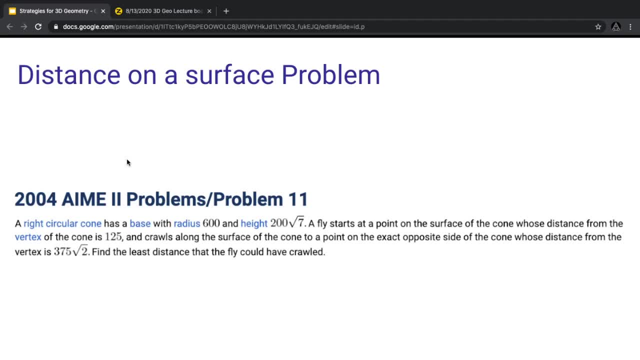 questions. of course you can just like gain membership, you just chat, whatever, and we also have a problem set that will come in the discord. so if you're not familiar with discord, you can just type it in the chat. and of course we also have a website. uh, if you guys are, my colleague could? 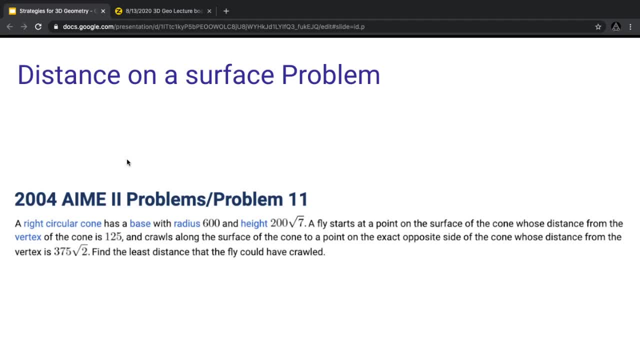 you guys put that in the chat please. we have a website and we have our youtube channel, which is where we post all the streams. okay, so first, does anyone have any? oh yeah, looks like they put the website link as well. you can find a lot of handouts we created on there too. 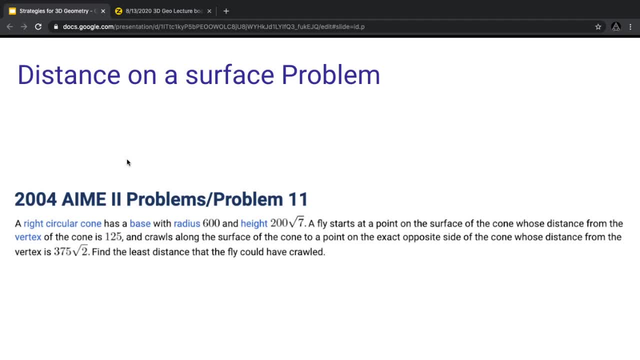 yeah, uh, does anyone have any questions? just please feel free to put it in the twitch chat, like if you guys want me to review any specific problem or any strategy, or you have like another 3d geo or anything, i'll feel free to just post it and i can walk you guys through it.